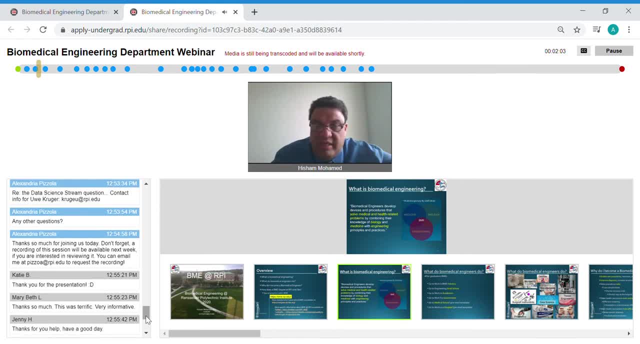 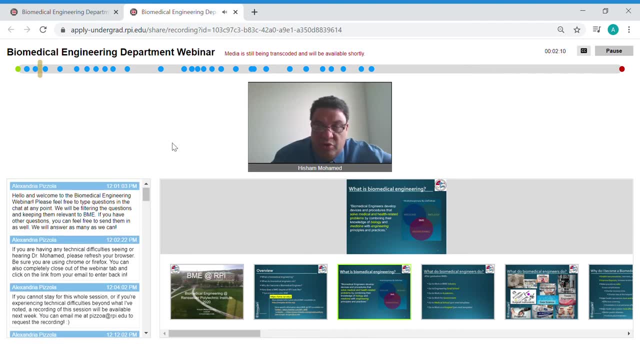 And everything that you find in a clinic when you walk in, everything that you see in a hospital or you don't see behind the behind the curtain, or anything that's in diagnostic lab that you go to that handles your blood or handle any of your brain cells in a relationship you're practicing and things like that. 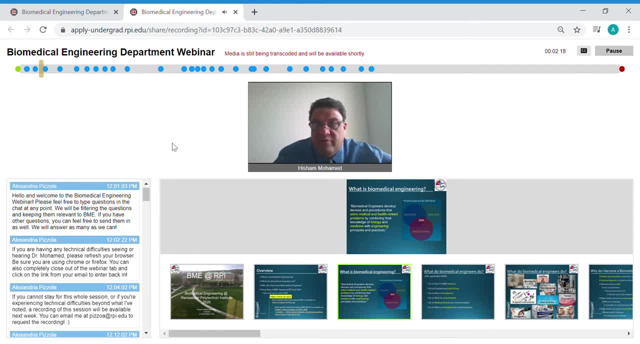 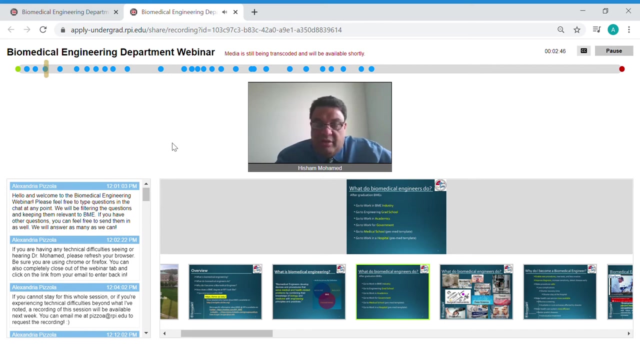 For the Bangalore it um worked in in for you Kps. So biomedical engineers: after they graduate they can go work for industry and there are multiple functions that they can do. They can be a research and development engineer, They can be working on other functions. 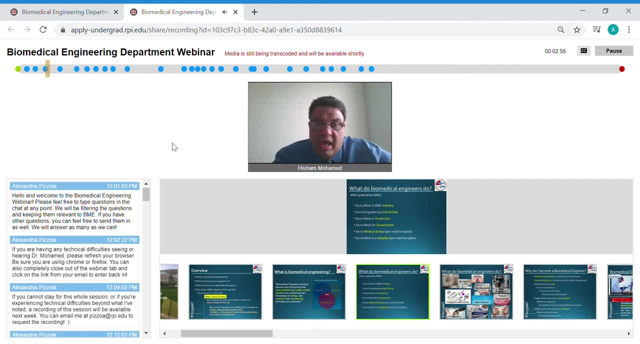 They can go to graduate school to have a master's or a PhD. After that they can go back to industry to work there to do research and development. They can go back to academia to teach and do research, or they can join a government, either a research lab. 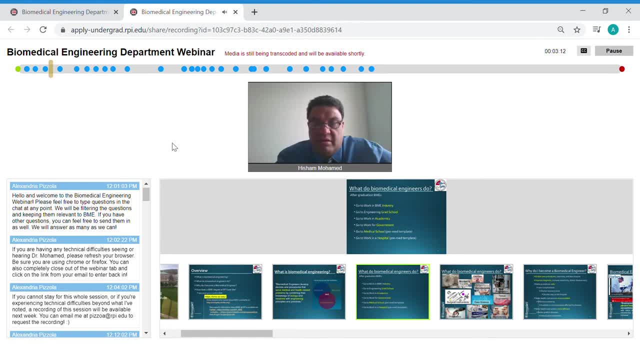 or they can join the regulation, like the FDA and other bodies that regulate the biomedical field. Many of the research, many of the great research, is done not just in academia, not just at Harvard and MIT, but are also done in government lab, on the federal level and on the state level. 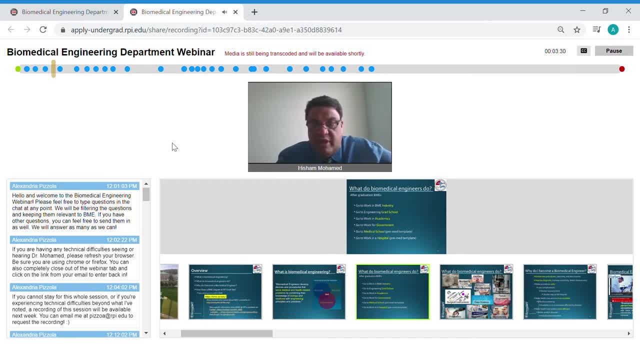 So there are a lot of opportunities to work also for the government, and they're a very good one. Some of our students choose to go to medical school, So they choose. we have a pre-med template where they can follow. I will talk about that. 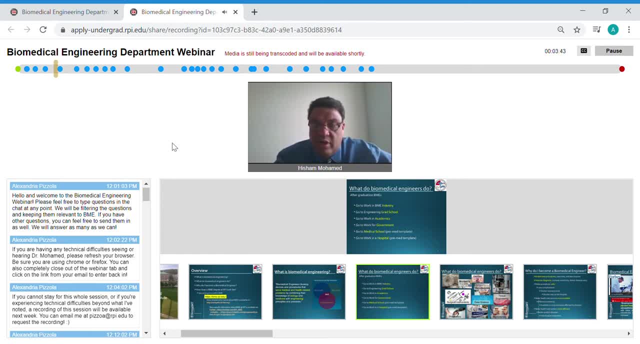 And some can work in the hospitals. They can work with- you know the people there- to design new imaging sequences or look at the images in a different way or do something different, develop something different, like people that are working now for the ventilators. 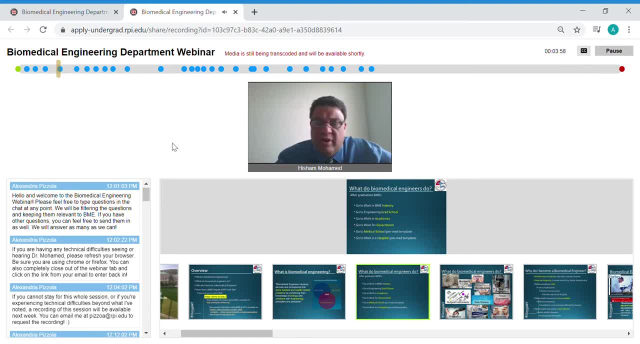 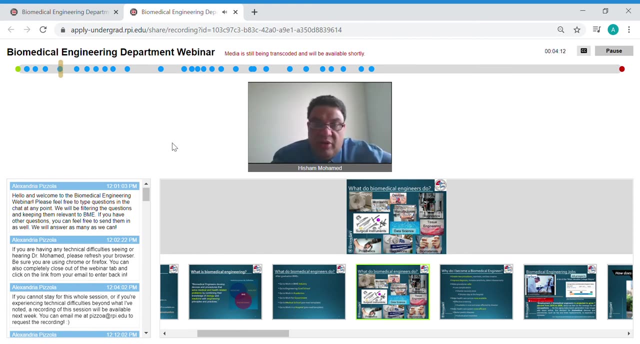 There are a lot of jobs also to work in hospitals, So there is a wide variety of jobs that you can do after you are done with your undergraduate degree. So some examples you have: you can work on imaging technique, monitoring all the equipment that's used for monitoring of ICU. 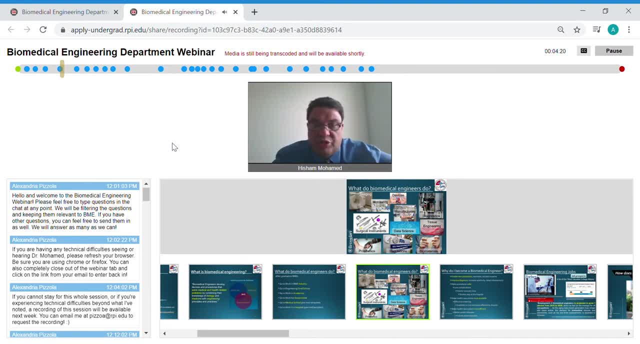 or after this implantable device, pacemaker, surgical instruments that goes in or used during the surgery, prosthetics, diagnostics- all of these falls under the falls under the device and imaging umbrella. It can work for manufacturing, too: Tissue engineering doing a mesh, for example. 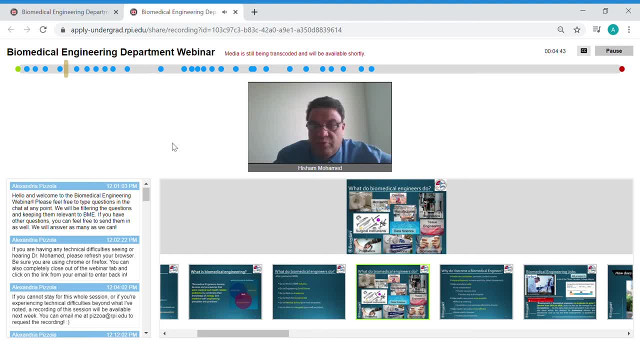 for hernia mesh doing for tissues replacement for burn victims. You can do also. you can work for the government, as I said, for regulation, for the FDA, And also you can work for a institute that does data science or you can work in data science area. 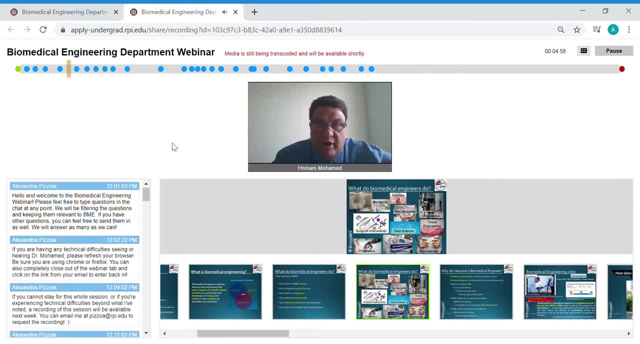 where we are trying to learn from data from previous experience, to try to try to predict what the future is, without a crystal ball, but using the data and experience from before. So you can see, these days, of course, data plays a very important role. you know who gets. 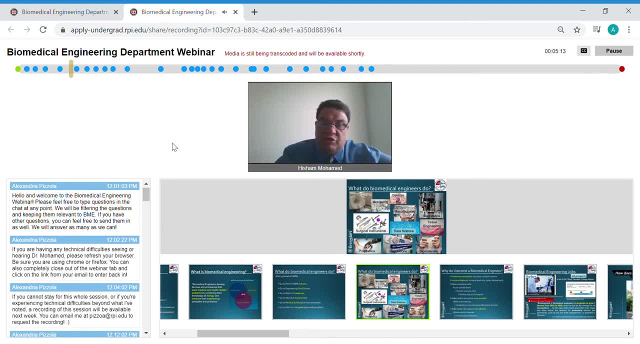 who gets infected when they're transmitting the disease? how long does it show on them before you know the symptoms show up after they're, after they are infected? All these are data that gets collected samples from different different patients. DNA. 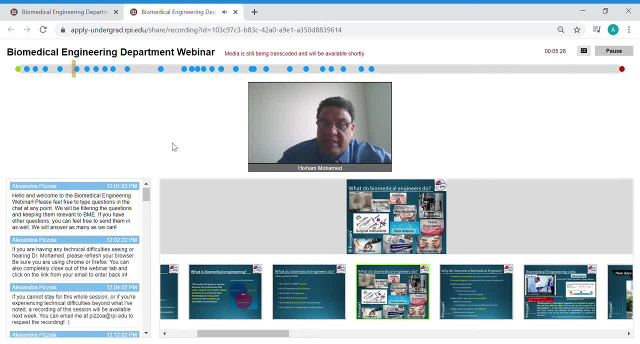 and these can be used in the future to predict how the disease progressed and how we can contain it and have a better way of doing this in the future. So all of these are. they resonate with the area of concentration that we have in our degree. 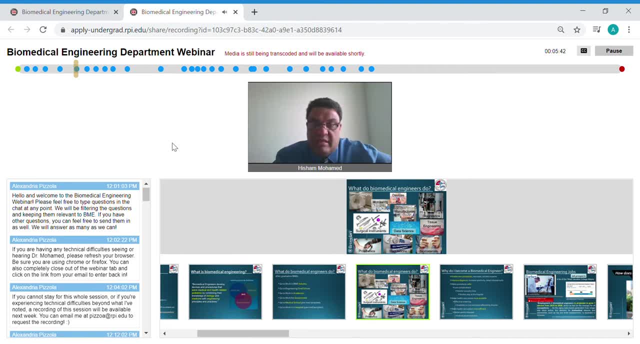 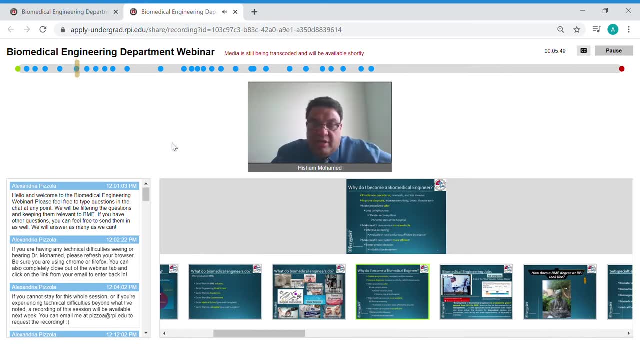 Imaging devices, biomaterials, data and so on. So why would you become a a biomedical engineer? We work, as I said, on new procedures. try to improve diagnostics, make it safer, make people stay less at the hospital. 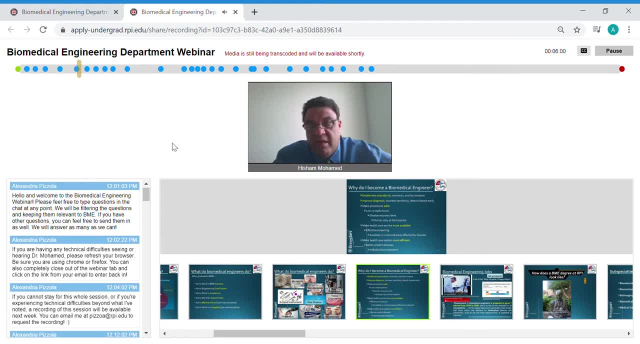 make people come back less frequently, come back, have issues with their, with their surgery or anything else less. You try to make service, health service, more available. It used to be hard, hard seal before that, but now everybody understand how availability is important. 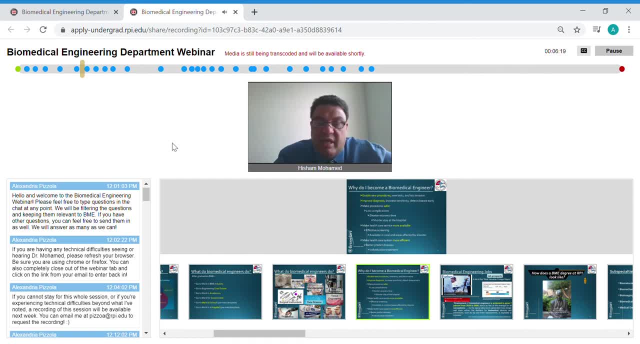 how to have availability of test, how we can things can be done quickly, how we can get the test back in a day or in hours instead of a day or two. So we try to make healthcare system more efficient, less expensive. It takes a big bite out of our GDP. 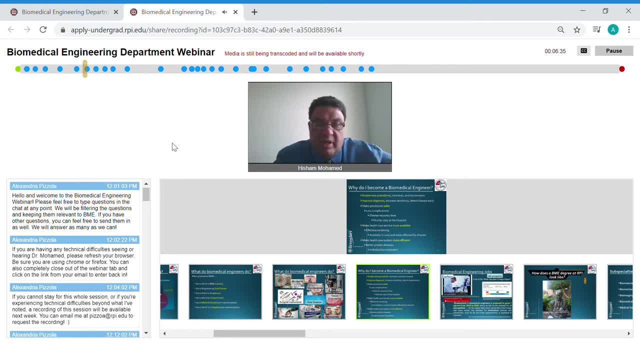 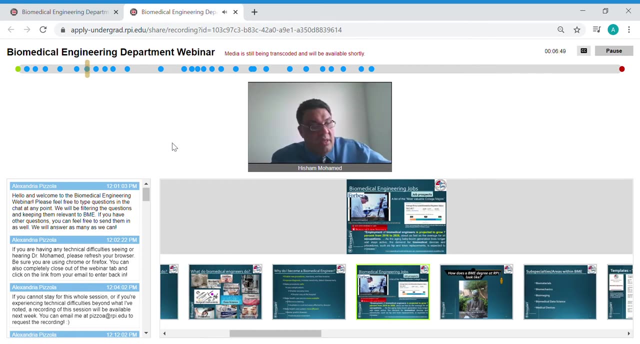 So if you can make things more more efficient, people come less back to the hospital. people need less treatment Or they need less pay at the hospitals, that will will help save on the on the grand scheme of things. So it's it's it's a good job. 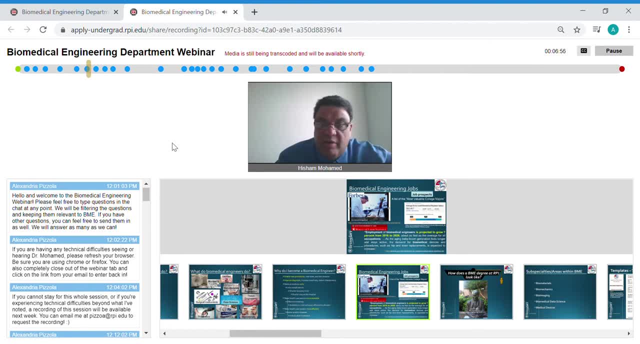 You can go out and see the numbers for the salaries. Biomedical engineering is a good job. It's a growing field. It grows six or 7% every year, predicted for the next 10 years or so. The one thing I'll add here: 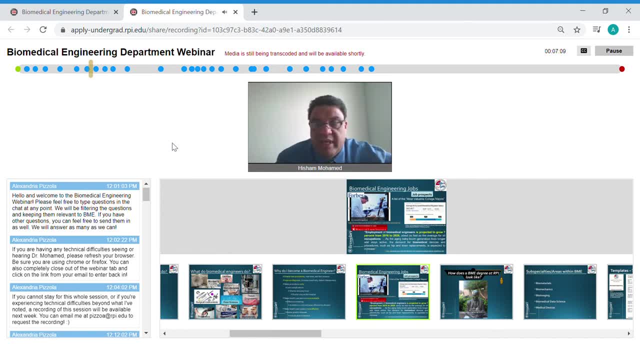 you can find all kinds of statistics online that will tell you how rewarding that is, But the one thing that I will tell you: it's a very satisfying job When you work for a company or a new treatment, or you are doing a new discovery. 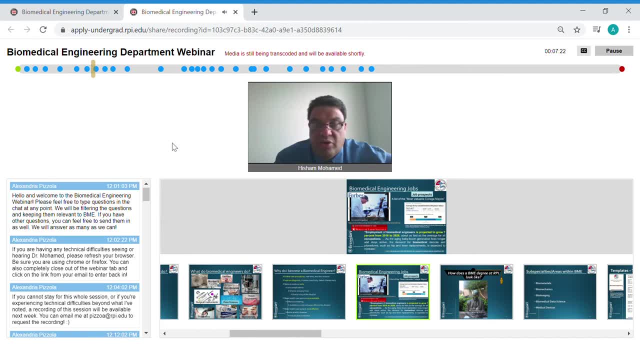 or you're going and applying your device on a pig or an animal and see what, the, what the results are. It's very rewarding and satisfying job, not just for the pay and for the for the goal, but for sure there is no shortage of jobs and they're good paying jobs. 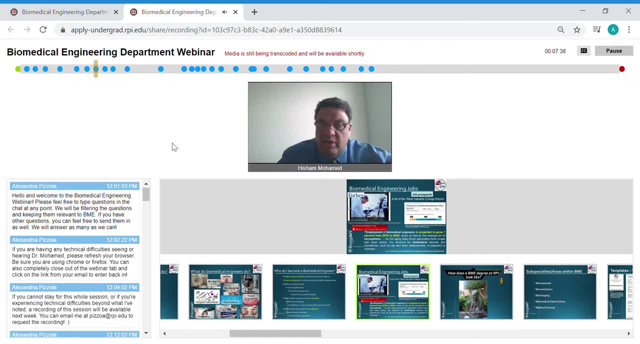 So let me. what I'm going to do here is I'm going to show you, I'm going to show you, I'm going to show you, I'm going to walk you through a little bit- If what a degree will look like at RPI. and this picture. 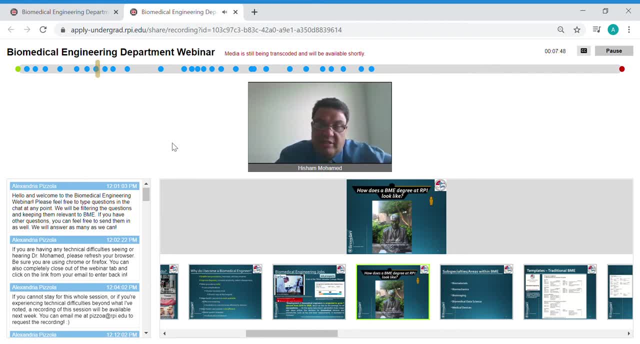 if you have visited campus. this is Dr Johnson. He is. this is statue in front of the building GEC, the Johnson engineering center, And it's named after him. He was one of the founder of a company that became after this Texas. 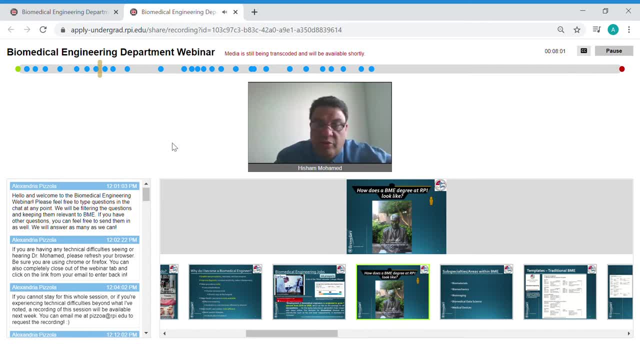 instrument. He's an RPI alum and you'll see his statue as you're going into the building. And the one thing that I like that in the summer, as you can see, people have put a sunglass glasses on him. in the fall, 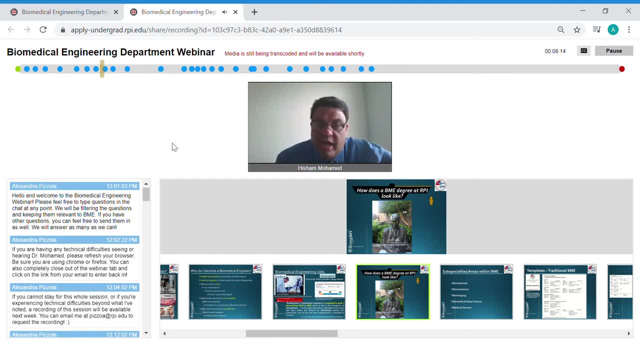 You'll see that sometimes students will dress him with a scarf Halloween. they'll dress him for Halloween, So he's kind of like a living thing. with us was every, every semester And they take some pictures for him when the students do that. 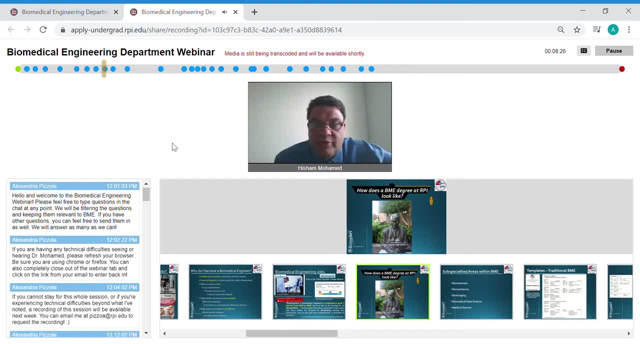 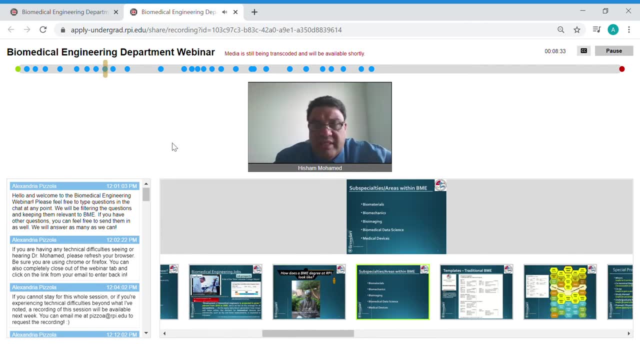 So I can share this picture with you later. but he is a part of our culture and part of our place. So let's talk about degree a little bit more specific: What's at RPI? So, as I said, we have five concentration areas. 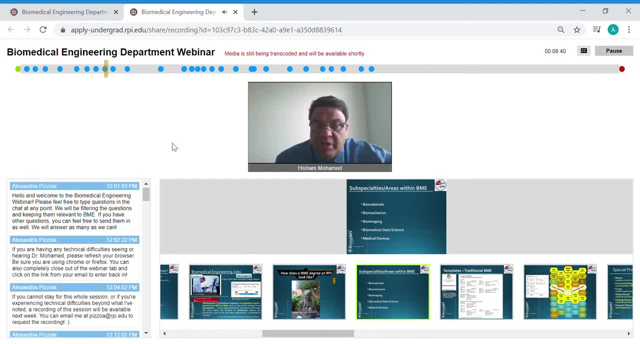 biomaterials, biomechanics, bioimaging, biomedical data science and medical devices. And biomedical data science is a new area that we have added this year. We used to have a bioimaging and bio instrumentation that we divided into because we 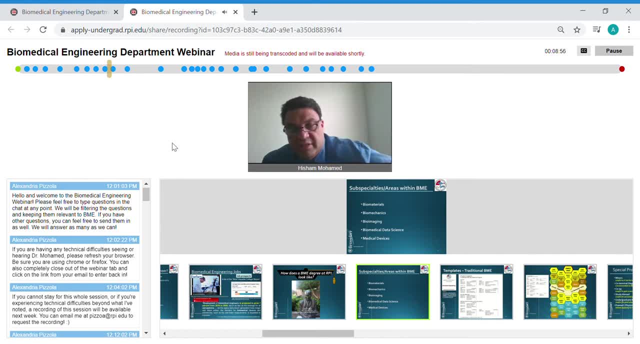 we saw the need of having more medical device areas. So the students can pick any of these and it will be on their degree as their graduation, at their graduating, that they have what area of what area of consultation they have And, of course, that coursework. 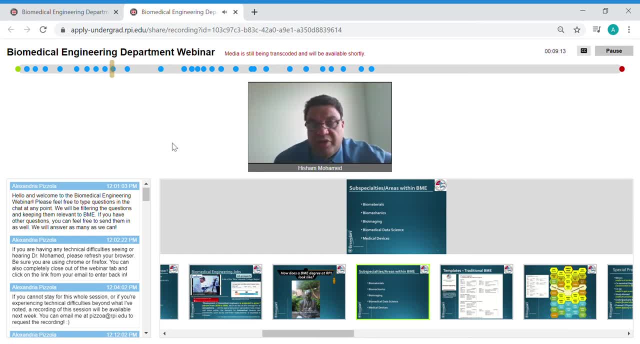 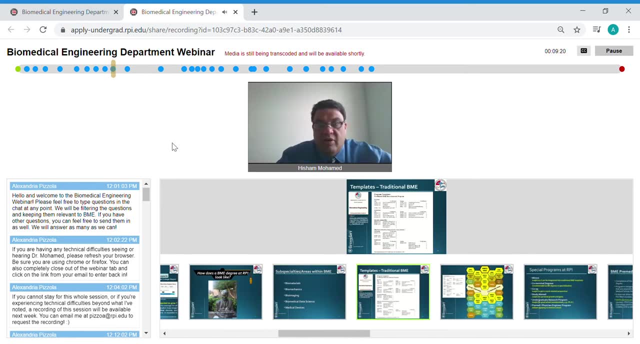 there is coursework that everybody takes, And then, when they think that concentration, there are a another, another addition to that. So this is how our degree template looks like. It's dry, I'm not talking about it much. It tells you every semester. 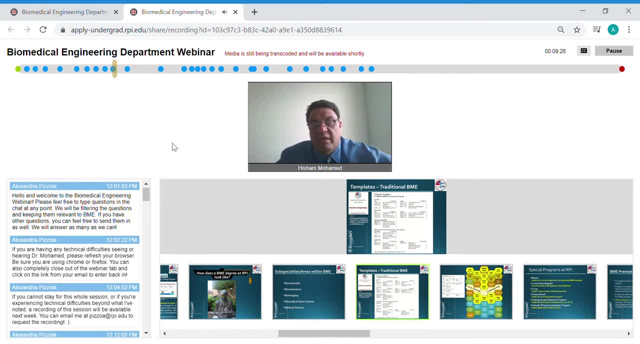 what kind of classes you are taking. It tells you what the sequence is. It's very important to follow it as closely as possible, because first, the some classes will be a prerequisite for another class, So you have to take them in order. The the semesters are very well designed for a balance of load, and 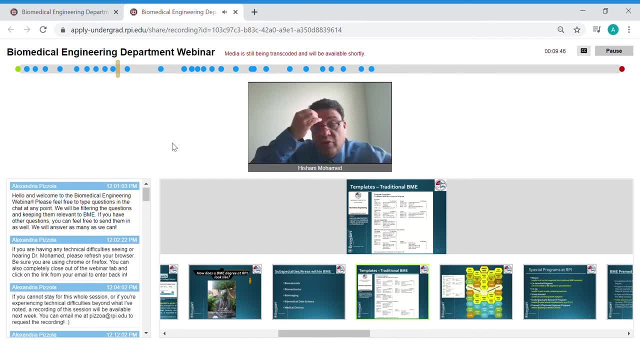 preparing you for the next phase, And the schedule also is is designed so you don't have conflict in times and you can take all these classes together. If, for any reason, you you diverge away from this template, that you might have if you keep a class that you're supposed to take the first year or 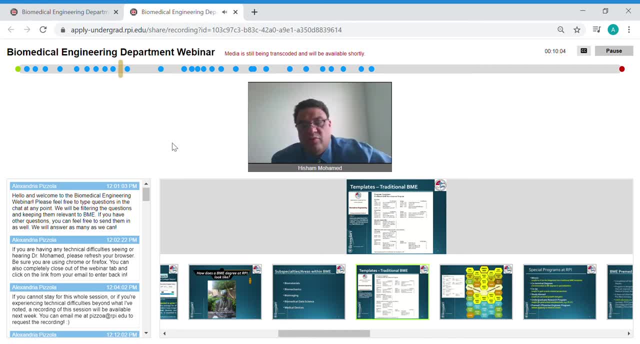 second year to the last semester, for example, you might have hard time scheduling because it was not meant to not overcome with the classes on the last year. So I would encourage you all to follow the template as closely as possible And if you diverge from it, 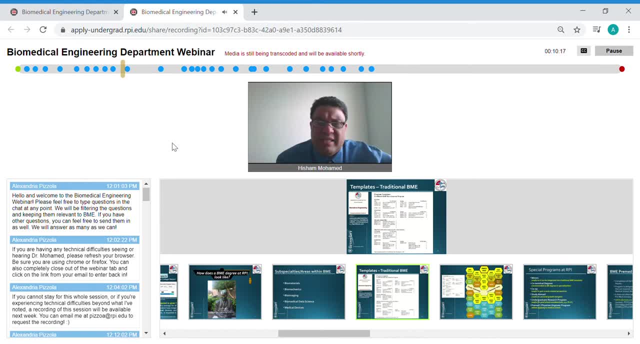 try to make it, keep it to minimum, but the template as is like this. it does not show you and your advisor. of course, your academic advisor can help you navigate this and work around it. Of course you might have some transfer credit. 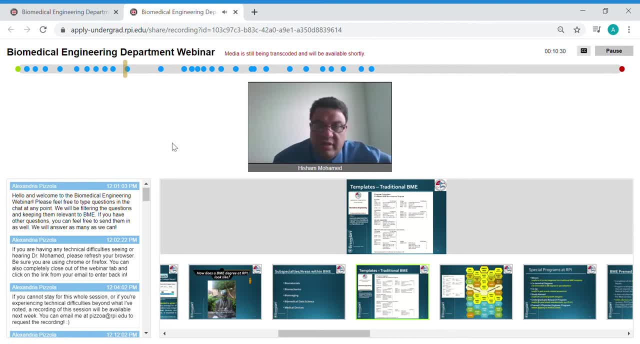 You might have taken credit somewhere else. So there are all those kinds of other scenarios where you you don't follow this exactly, but try to follow as close as possible to maintain the load too. So a better way of looking at it. I like to look at it as that way. 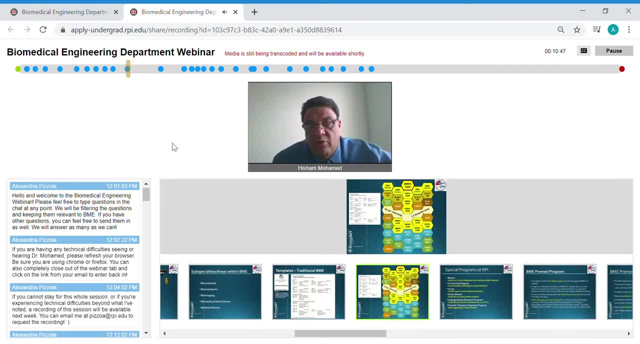 So instead of going top to bottom, semester by semester, I will go bottom to top, And in this one I would like to- so you can see that you start with some basic classes- engineering, math, biology, physics and so on- So you can have the basic. 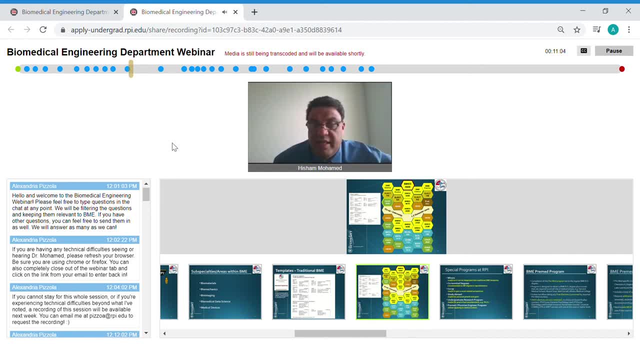 The first year is mainly the foundation of this And then you can see. starting from the second year, you start seeing off a P yellow. a lot of biomedical engineering classes, And the one that you start with are meant to give you the breadth first. 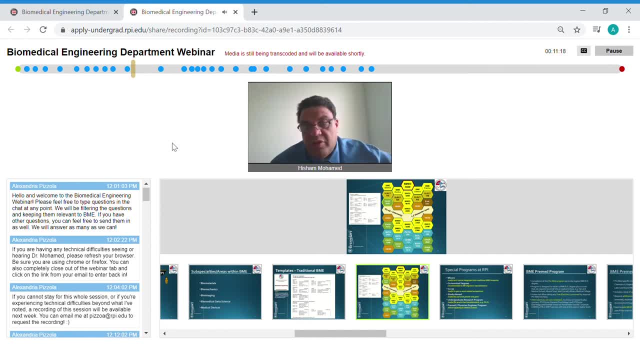 So you have one for biomechanics, one for bioimaging and bio instrumentation, one for biomaterials and one for data science. that will prepare you for this. So these four will cover the five areas, And then you have a more on the modeling of biomedical systems. 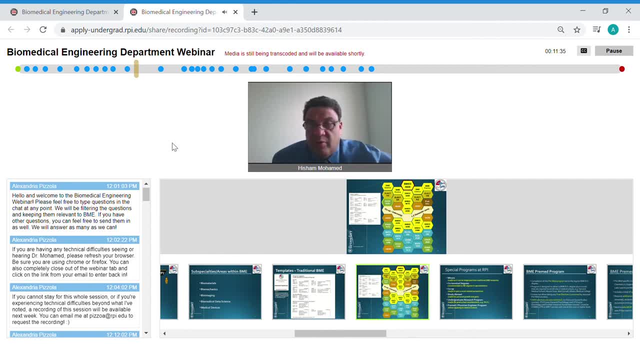 and you have also more engineering, where it's preparing you with a professional development component. so you are, you have the breadth of your knowledge after the second year. you are kind of understand where we are going with this education And before you go further, 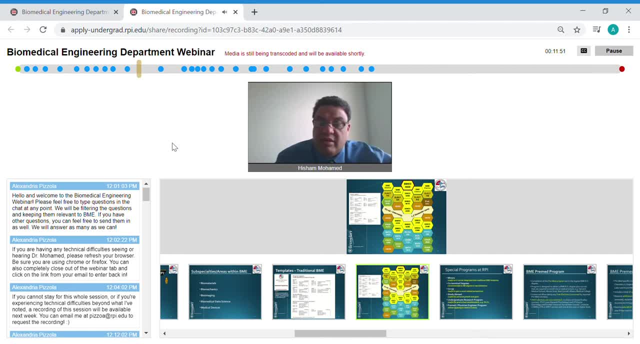 we have the. we have the summer arch where you can take. you can take classes in the summer and be away for a semester or two during the year. So by doing that you can have a corporate internship where you go out after you have done two years in school. 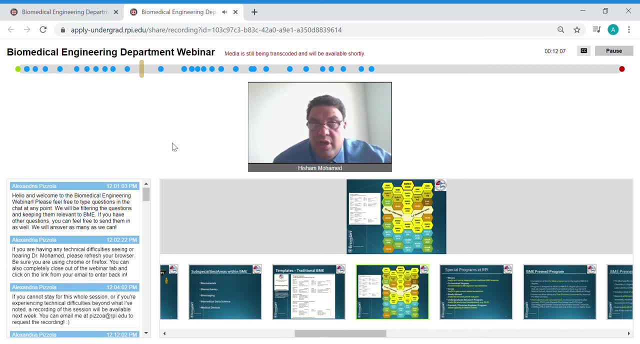 and now you are ready to go and explore. What do you want to do Now? I understand what biomedical engineering is. I understand what the different parts of biomedical engineering is And I would like to explore the. you know, go work for a company or work for a startup or work. 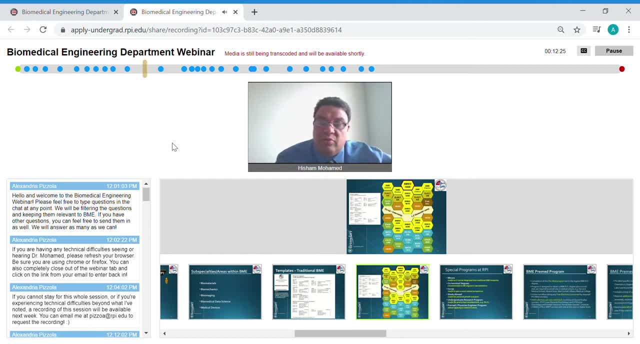 for a lab and see how things are, And that will help me make my mind when I go forward with this. Then they come back from the co-op or the internship once a semester or two semesters away, And now they're ready to. 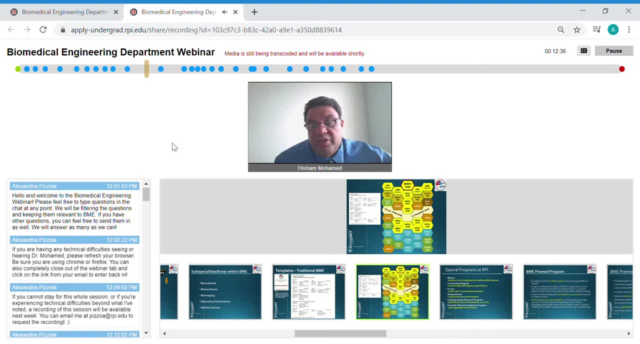 for the next year and a half to finish Now. now they come back to advanced physiology, For example. this is one of the one of the one of the star classes that we have where they can do dissection on pigs and they can do small procedures. 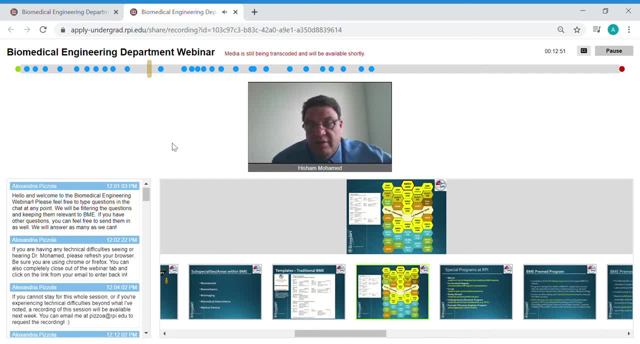 So they have hands on with Albany med, which is a the biggest hospital in this area, Albany medical center. Then they do the lab, where they have hands on experience on how to do mechanical testing, how to do tissue, how to do other parts. 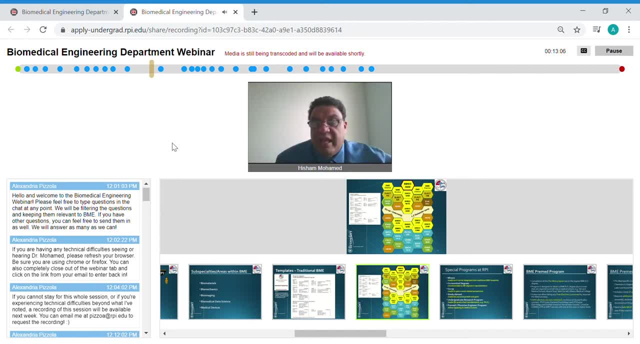 imaging and so on. And then they have- they have that Elective. You can see that they have four or five electives and they have- these are free elective, that they can increase the depth of their knowledge in any area. And then they have the biomedical elective. 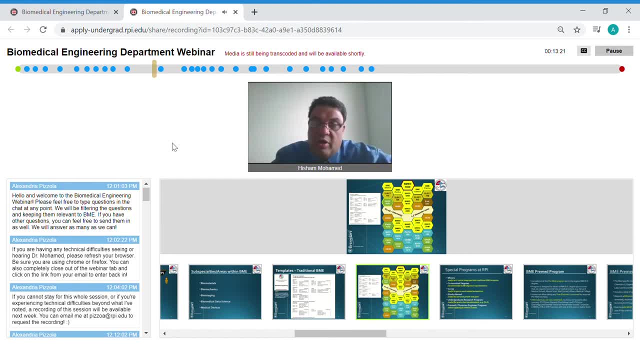 which is the depth in whatever area they pick, by materials or biomechanics or so on, So you can see after they come back. they now, they have the knowledge, enough knowledge to tell them to start shaping their own education and where they go. So they get the breadth from the first two years or so. 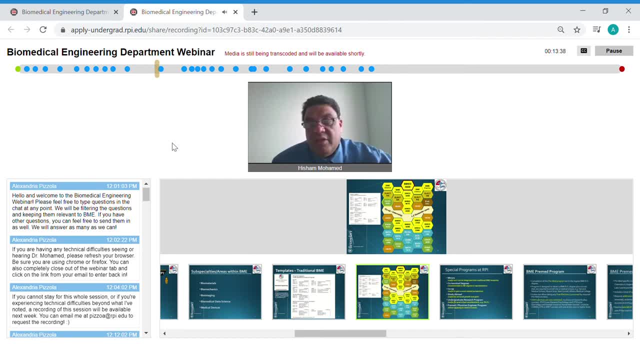 and the solid foundation, solid technical foundation, And then the last two years they shape it where they have the depth in what they want to and maybe some breadth is they want to add to. So they have a stay in their degree and degree is very. 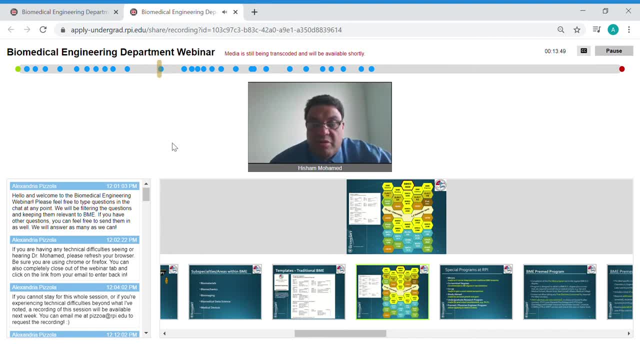 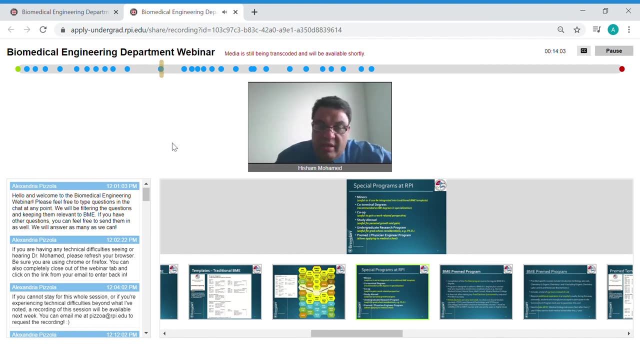 well designed to bring them. when they're out of this, they are there to go and join grad school or any place that will be very competitive when they're out of RPI. So we have- you can have- a minor. many people will have a major in biomedical and a minor in. 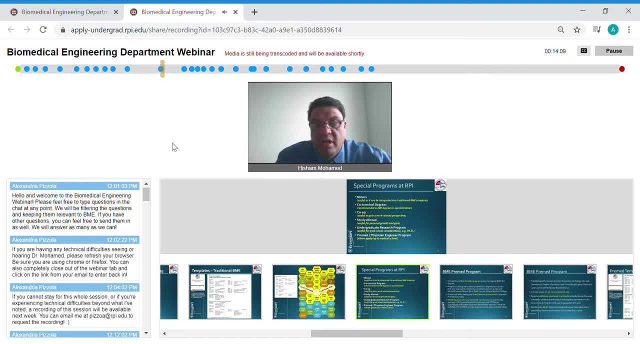 in other classical engineering like electrical or mechanical. They're useful If you want to do that, if you take enough courses. there is a co-terminal degree also, where you can stay a fifth year after you finish your bachelor and get a master of engineering. 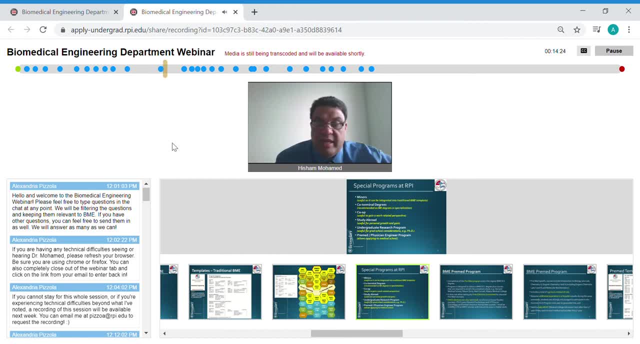 Many of our students choose that, So they have more depth in the area that they want. And we have co-terminal as engineering and RPI also offered co-terminal as a mix between engineering and business. You can talk to the business school. They have a good program for that. 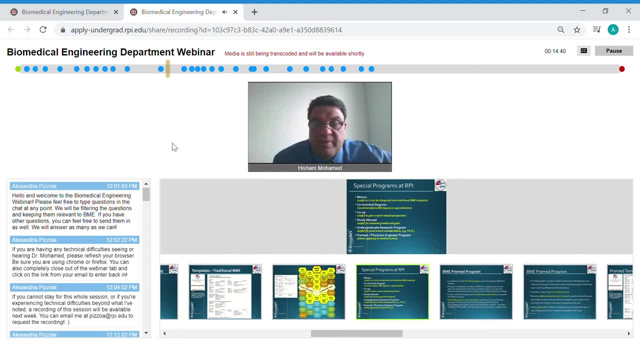 And there are co-ops help. you get co-ops So you can get the experience after the second year where you can have a better choice of how to pursue your degree. After this there are study abroad programs where you can go to France and go. 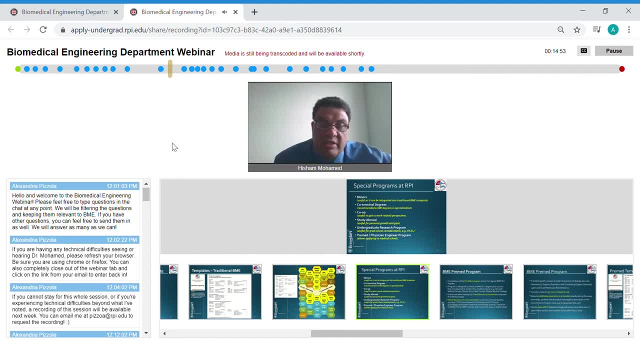 to other places, work in the research lab or take classes somewhere else. It's made to your. I mean an engineer is a, I mean it's a person that you need to diversify their skills and their the things that they know. 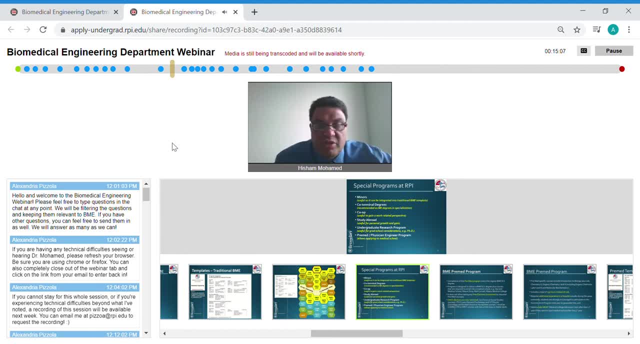 So it's not just the classes that they take, but how other culture deal with, deal with problems, how they, how hospitals are running other other places. What are the regulation from one country to the other, the U? S and Europe and other Japan? 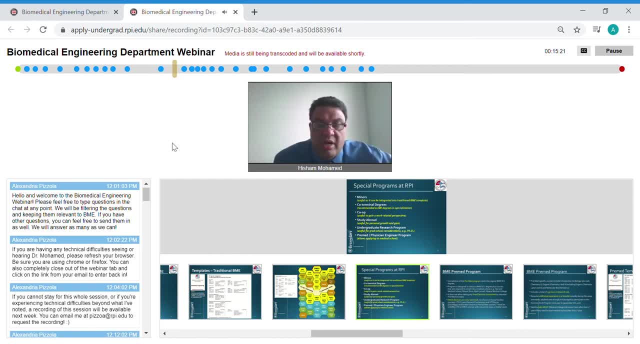 for example. So this is. it's meant to make them a well-rounded, So when they're, when they're in industry or they're tackling a problem, they know what the issues that involve in this. There are other graduate research programs at RPI. 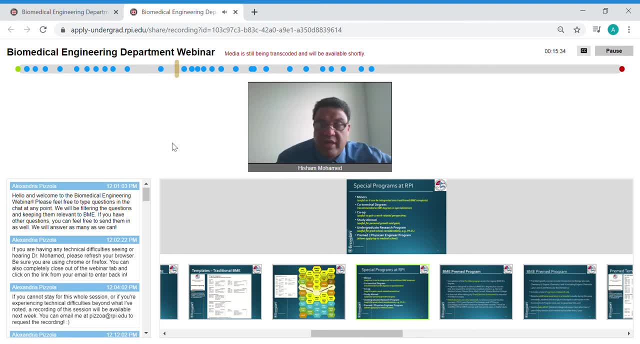 They can join, for they join and do research with any of the faculty that does research at RPI, And we are proud to say that almost 50% of our students have a search undergraduate research experience And this is very useful if they're going to go. 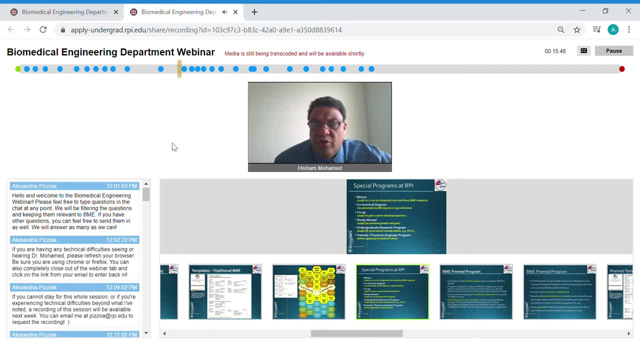 for example, for grad school after them, And it's useful in general because you go into the lab and you're working with a problem and see what the issues are, And there is a pre-med and physician engineer program that I will talk about. 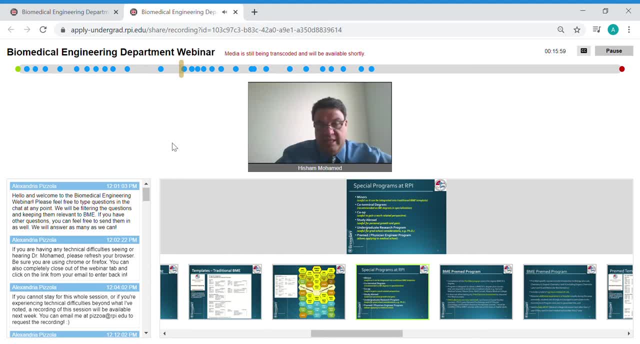 Pre-med is to prepare you for going to apply for medical school, And then the physician engineer program is a little bit limited in number, but allow you to be four years at RPI And get a bachelor, And then four years at Albany medical center and get an MD degree. 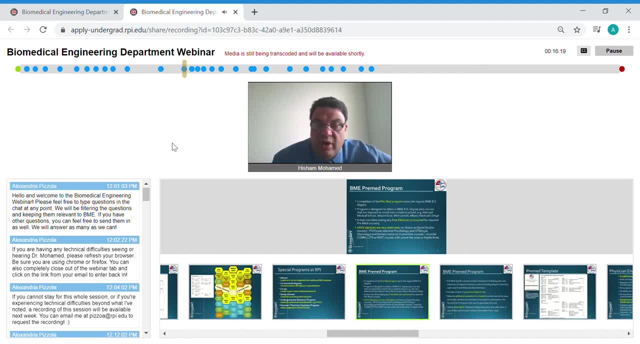 So the pre-med program is meant that you take all the requirements for the medical school. It's the one thing I'll say. it's challenging. You have to keep a GPE Most of your free elective that I talked about in the last slides. 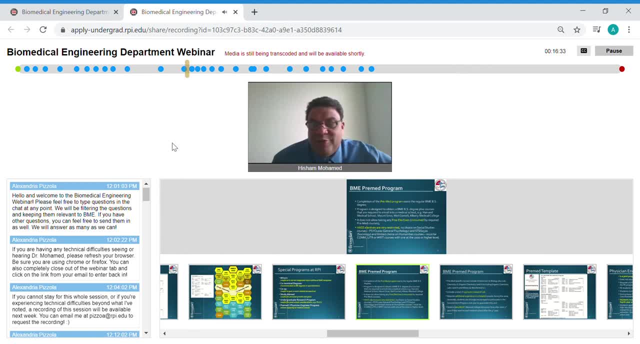 are not free anymore. You have to take that, consumed by some of the required pre-med programs, Pre-medical, pre-medical courses. the same thing for the hearts, for the human and the human courses, human and social science courses are- are also taken for. 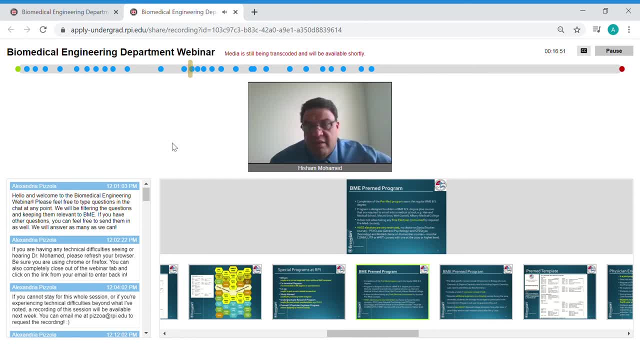 to meet the requirement for pre-med, but there is a, there is a template for it And we have also two dedicated advisors that will help you navigate this template and help you when it comes to apply for medical school. Also, it has requires a little bit more. more, more credit hours than than the usual. it's. you have to have some experience on some additional program that you have to join with Albany med or join in hospital, And then you have to take the MCAT after the third year to be able to. 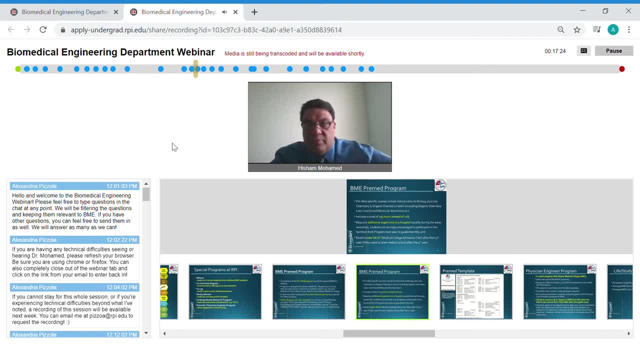 join a medical school after the fourth year. So it's successful program. It's many of our students forward. It's very good. The only thing, as I said, you lose some of the freedom for the elective and you have to keep your GPA. 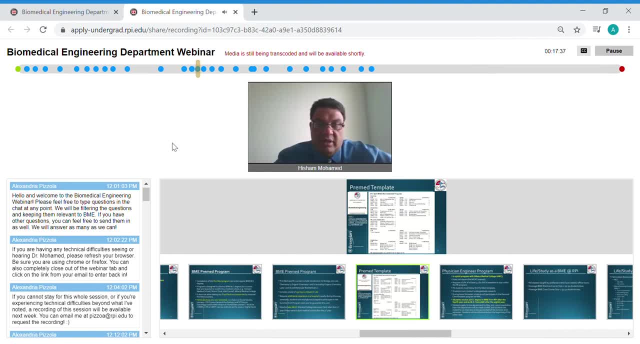 And we have a pre-med also in the in our our book that will show you what, what classes to take and what semester. And I don't think you remember from the previous template, but from the previous template we had a lot of things that it says elective here. 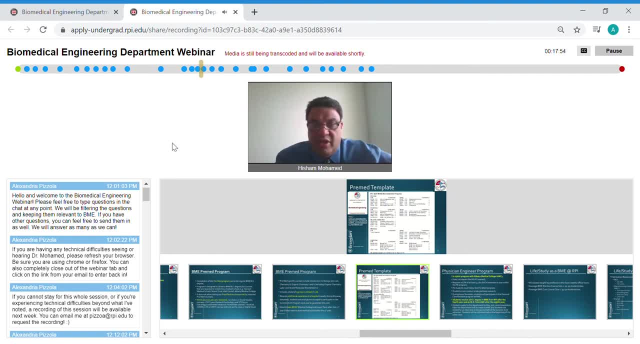 or you can take this, or free elective or free BME elective. You can see, on this template there is very limited free elective or free courses. Most of your courses are designed for you So you can meet the requirement for the biomedical engineering. 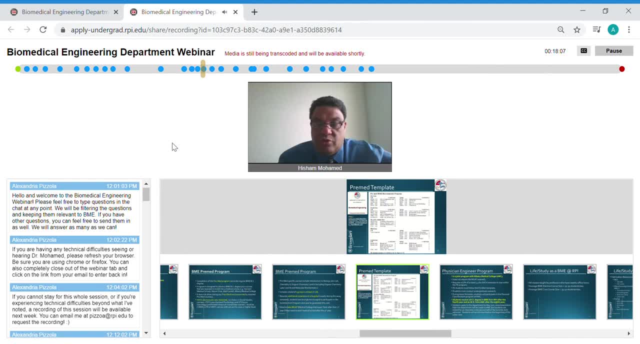 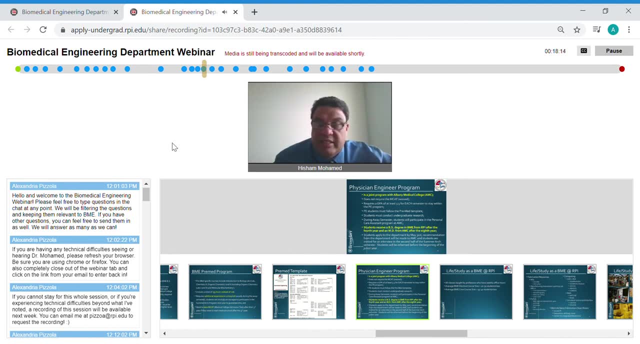 So if you're a bachelor and two for a pre-med to be able to apply to a medical school, the physician engineer program is, again it's a program. This one is done joint with Albany med, Albany medical self college. The one thing here, that's your MCAT is waived. 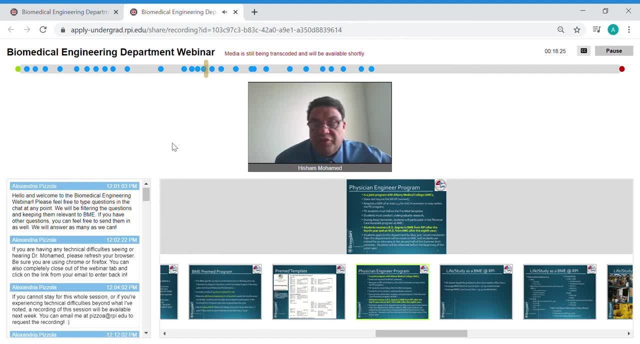 If you go through this program and you keep a GPA of 3.5, then you stay within the physical engineer physician engineer program And again you follow the pre-med template And you have, after 40 years at RPI, you receive a bachelor degree from RPI. 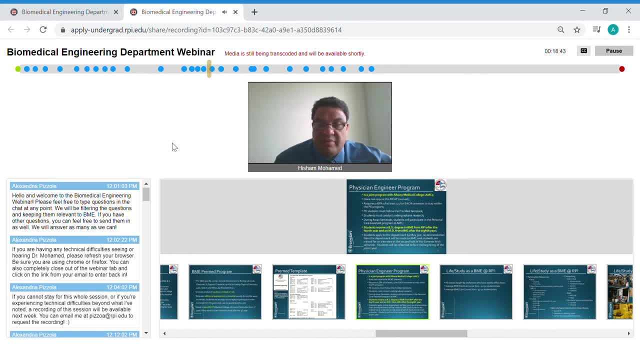 And then after the eighth year, you receive a MD from the Albany med. students apply to it. That is data When you get. if you choose to do that, I will ask you to talk to the two advisors for the medical school and they will walk you through this. 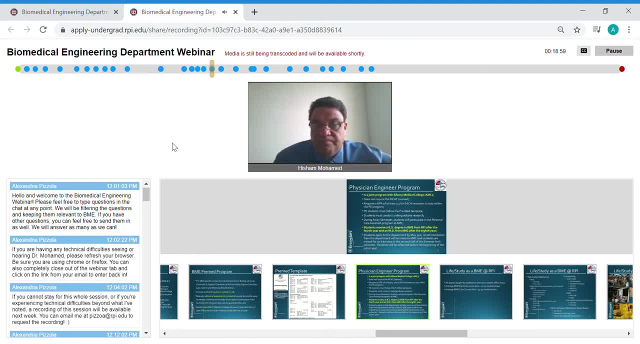 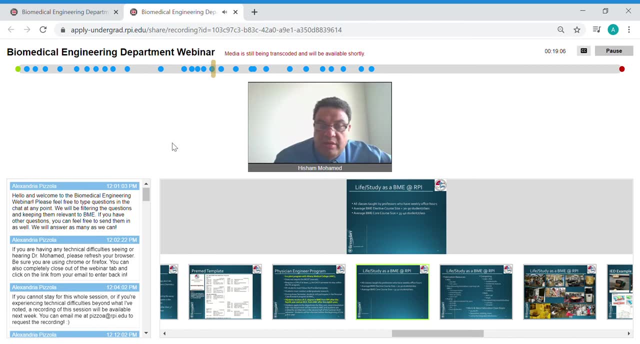 Some details. It's too much to talk about it here. In short, we we try to keep our our courses to be to be limited in numbers, So our elective courses are usually 2025. students up to 30, our core courses 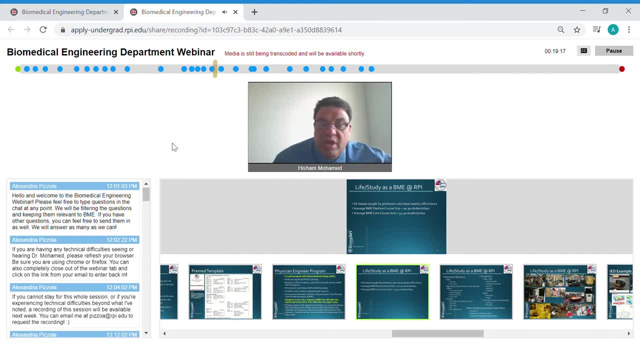 They are in the 40 thirties, upper thirties and 40 range. We have all professors have weekly office hours. We are all clustered in two locations. That's easy to access and easy to talk to professors. So it's always a good relationship between the professors and and the 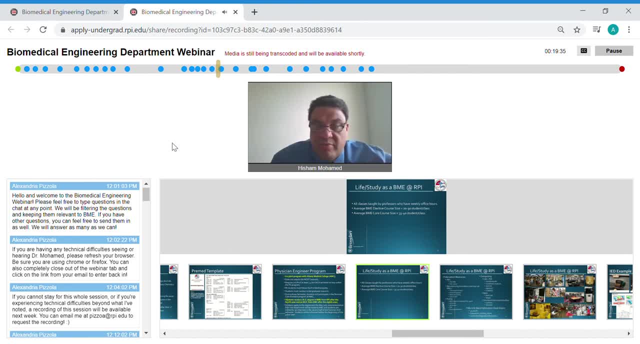 students And the one was good- Good memory. I don't have a very good memory, but the one with good memory remember every name of the of the entire class. I'm still struggling with that part, but it's always meant for the students to be able to. 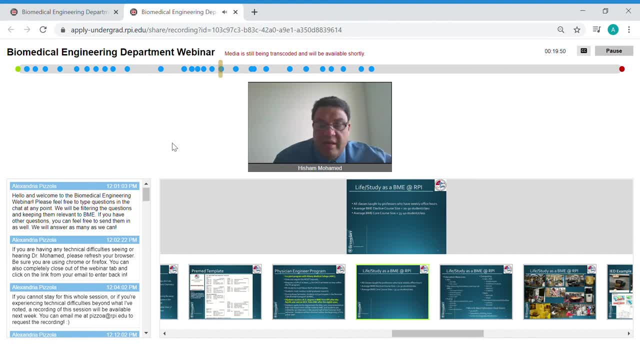 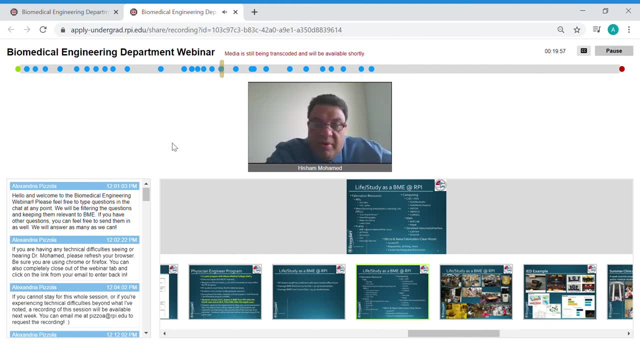 have their question, answer, feedback and get the best out of the materials. We are preparing the students to be engineers. We are preparing them to be designers for the future solutions, So we try to enable them with all the, all the capabilities that might need. 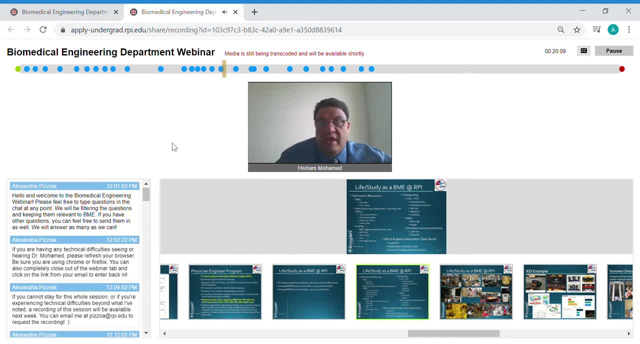 So we have a lot of application resources spread around campus. We have a manufacturing innovation learning lab, the mills. we have the MDL- It's another facility- And all of these are multiple locations. in the GEC We have other location. 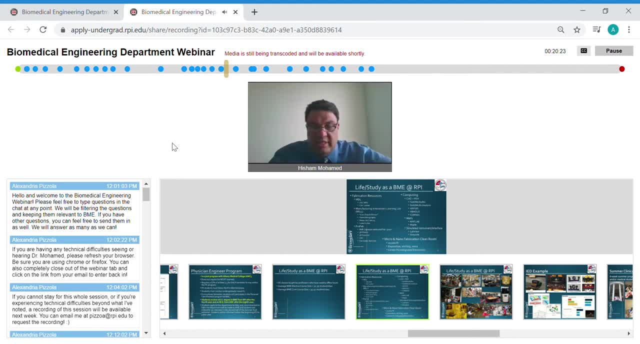 and then we have a profile that's designed just for, that's dedicated to the biomedical engineers. So when they do their design courses, their capstone, their the, they are, they are in yield And also we have all the, we have license for all the software that they might need. 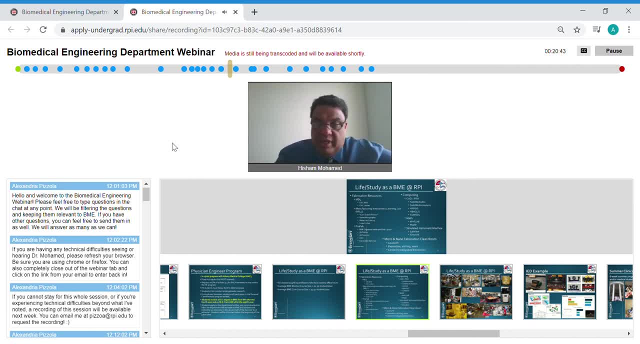 not lab finite element stuff like this, So they can do all the cross work and they can also design. We have also a micro and nano fabrication clean room for making integrated circuits, members, micro electrical devices and small devices like sensors. One of the oldest in the nation. 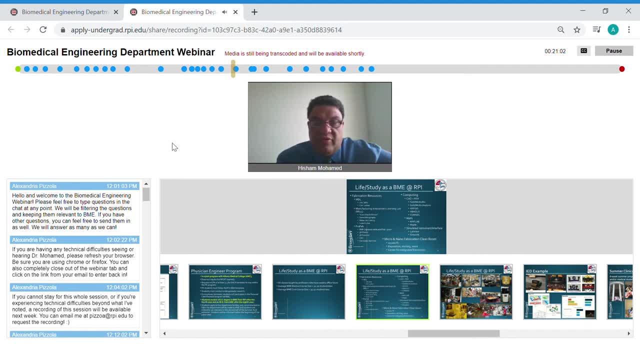 and it's very well maintained and get the students have a very good experience Doing this. I just realized one of the things that I missed to point out when I was talking about degree: that there are one of the things that we. let me go back to it. 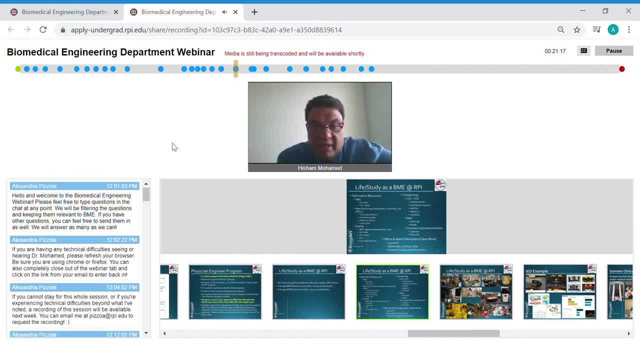 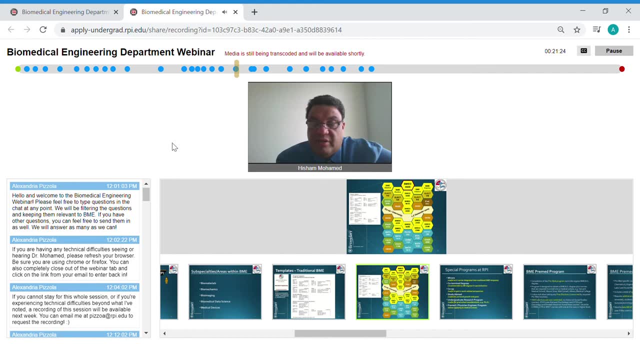 I apologize for that. I will go back to the slides because I missed a couple of points here. So when I was talking about this, so when they come back, we talked about their elective and their design courses. but two things I should have pointed to. 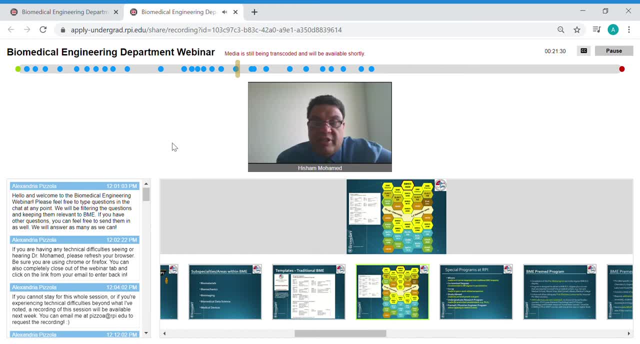 First, we have a introduction to engineering design. This is their first design course that they take engineering 2050. And they build something and they'll give you an example at the end. Then they take their capstone at the end, which is a sequence of two courses. 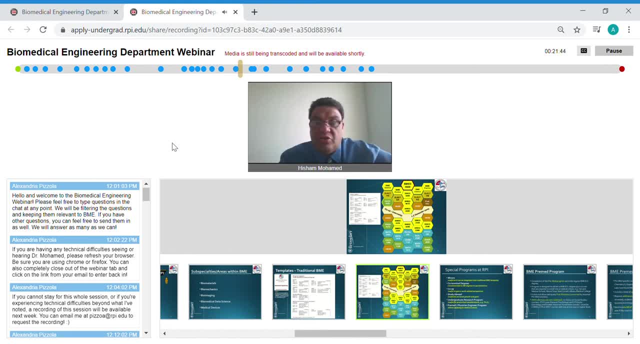 The last two, BME D 4260 and 4600.. That's their capstone When they do a senior project for that design. these projects are all coming from industry, from clinician and from a lucky center for disability and Albany. 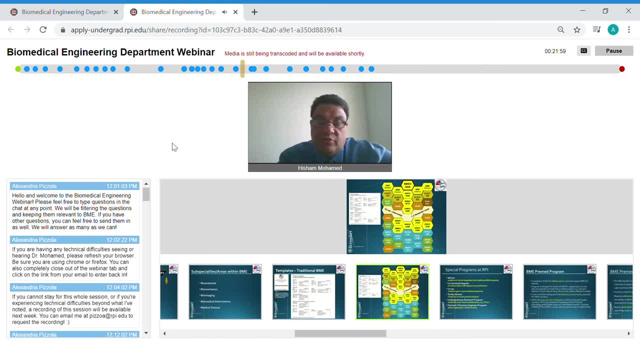 So are all coming from real problems and they prepare the students to work on a real, real, real world problem And and they have to interact with experts in that field And the other thing that we take pride in at RPI, that we have to design. 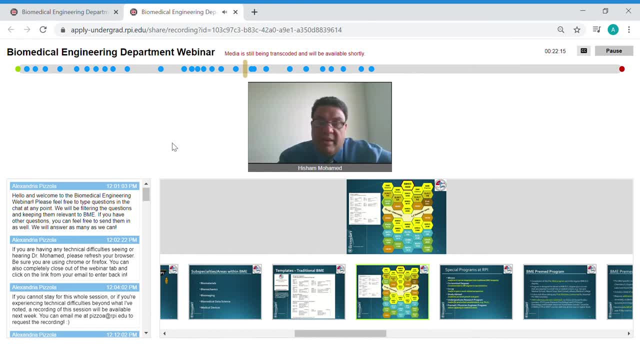 we have to design opportunities, not only a capstone, but the capstone and engineering 2050,, which is IED short for introduction to engineering design. That's very important to prepare the students, As I said at the end of the day. 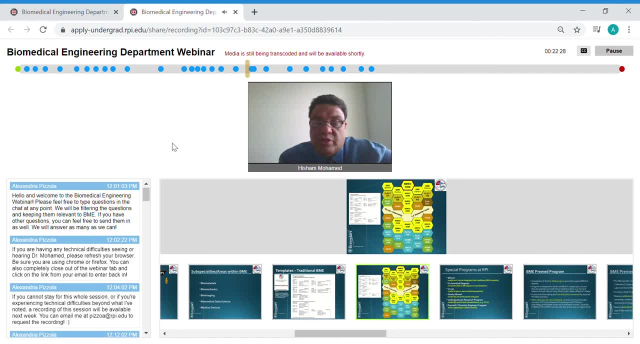 our students are designers. They get out and they design new solutions, and having two design courses it's something that we are proud of. Most of our school will have only one and might be only one semester. Ours is two semester plus this semester. 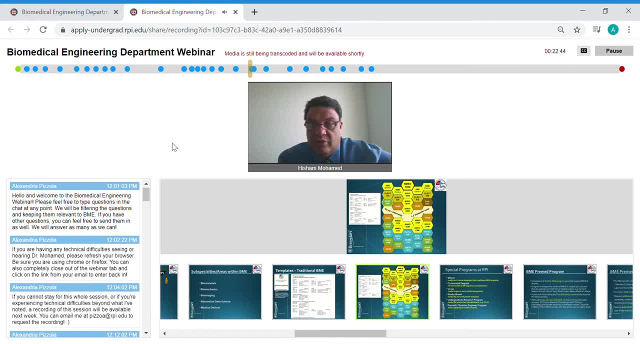 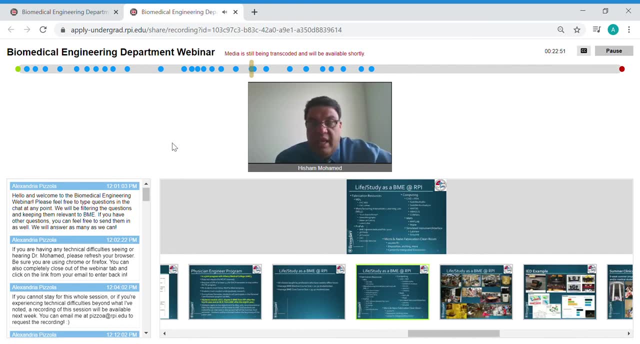 So they have three semester long design experience before they go out. So let me jump back to where I was. I just realized that when I was talking about the capabilities- and these are some of the picture of the facilities existing around the campus includes the BME lab. 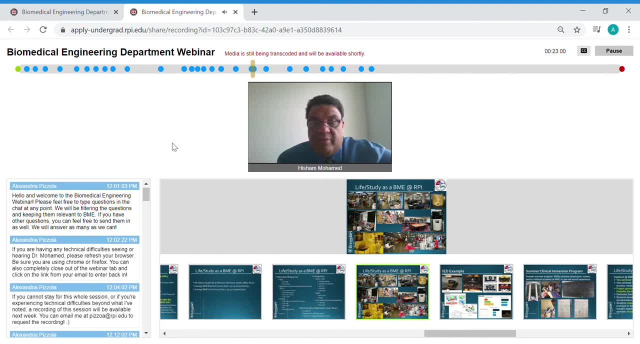 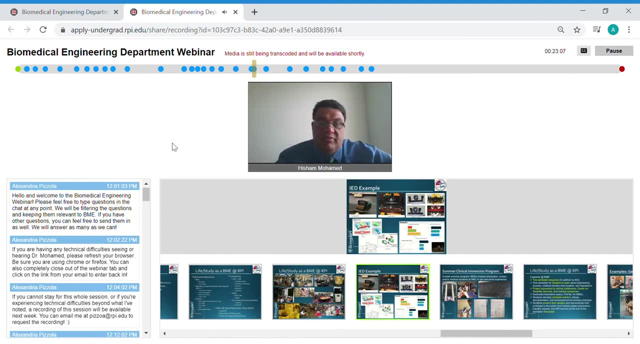 It includes: includes all the all the fabrication facility that will enable you to work on yourself Your solution. So I'll start wrapping here and start answering your question. Some of the examples coming from the IED, the introduction to engineering design. So the students in this class- 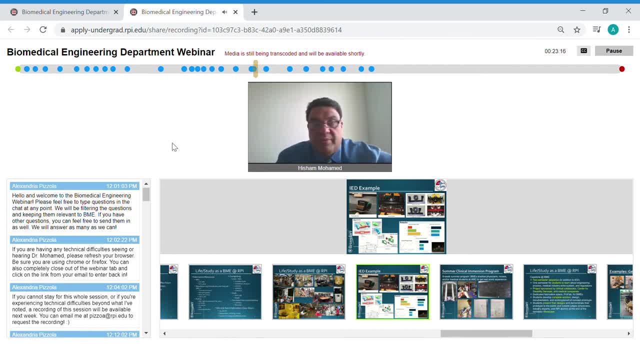 they pick their own project. They go, they build a prototype. So this was a control for a skateboard- make it motorized and control it. So they built. this was impressive. They built everything in metal. They went to the shop and they machined everything. 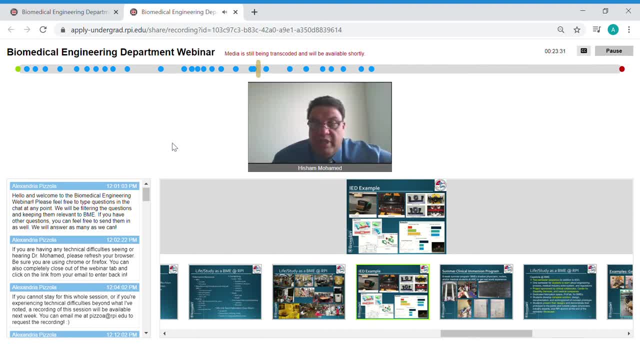 So this was the final material. They went through several design iterations. They went through several design iterations. They went through several design iterations To be able to to improve on this. They had CAD models, They had some simulation and they also had some testing results where they 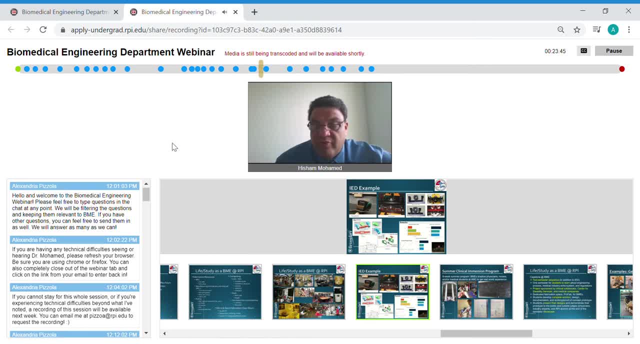 tested this at night. If you have been on campus, this is a walkway from the 15th street bridge to GAC- And at night they tested their system several times. recorded, recorded. And that's what engineering is about. You are. 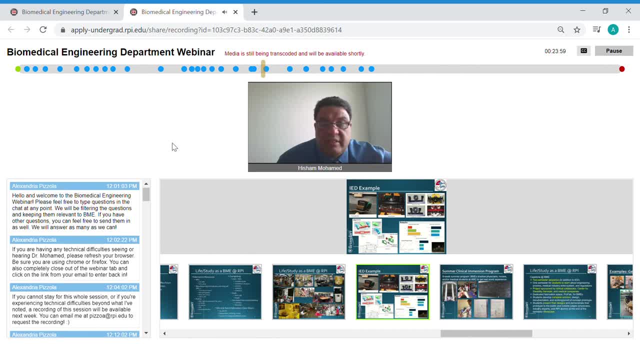 you have a unmet need, You have a problem that does not have a current solution, You go and you design a solution, You engineer a solution, You test it, You make sure that this is what it's supposed to be And then, when it's safe, 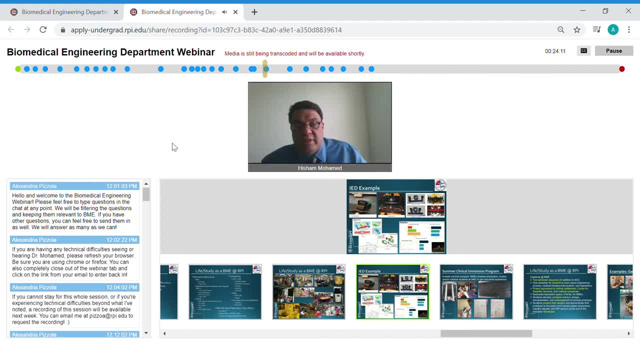 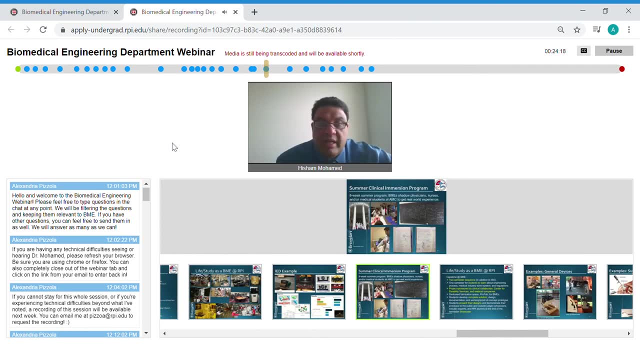 you can roll it out and they go through this design sequence in the IED. Another thing that we are also proud of: we have something called the summer clinical immersion program. This is a program, that summer program that runs for eight weeks with Albany medical center. 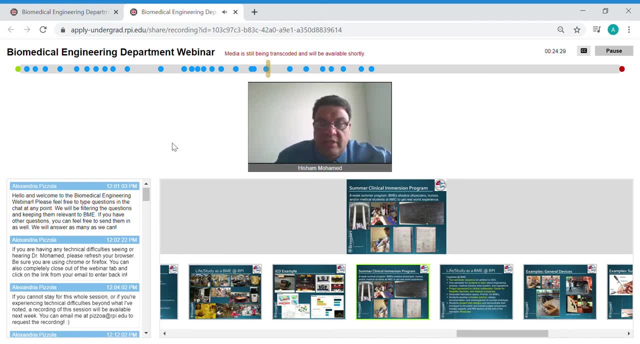 I oversee this. I oversee this program for the last two years, So we have a depends on the year, but we have a handful of students- six or eight- that they go and they spend six weeks shadowing doctors at Albany med. This is an experience that's unmatched anywhere. 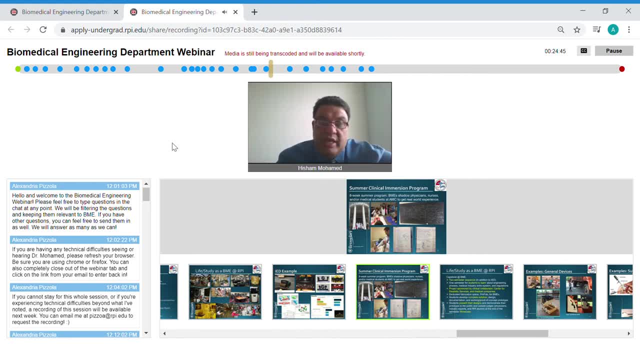 So biomedical engineer get to see how devices are used and to understand about the medical part of it, the medical aspect of it, So how things are used, how things are in the clean room, how patient care is and all the issues related to this. 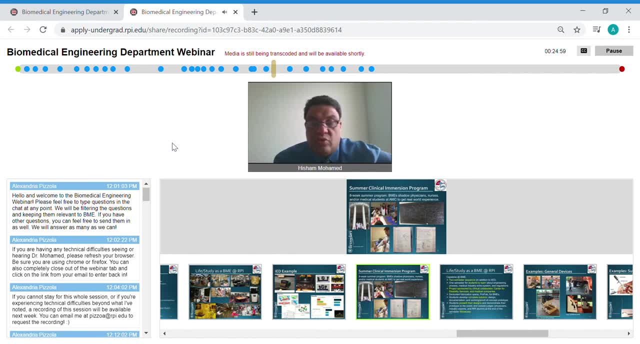 They spend a week at the beginning getting their training on how to interact with patient, how to protect their, their privacy and how to follow the protocols from the hospital- the safety protocols from the hospital- for six weeks. they shadow every two or three days. 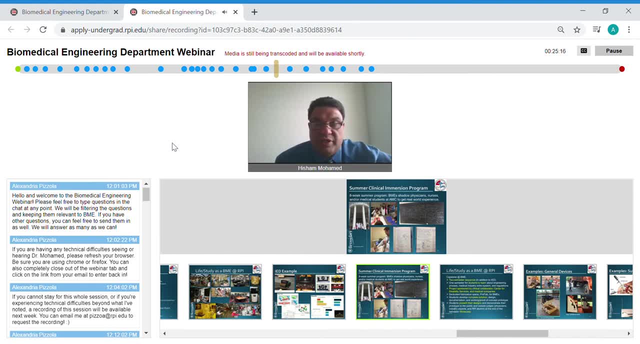 They're in different clinic, different in the operation room, attending whatever procedures are available for that day. They're separated in groups of two, So we don't have a big group in one or at the time And then at the end of the day. 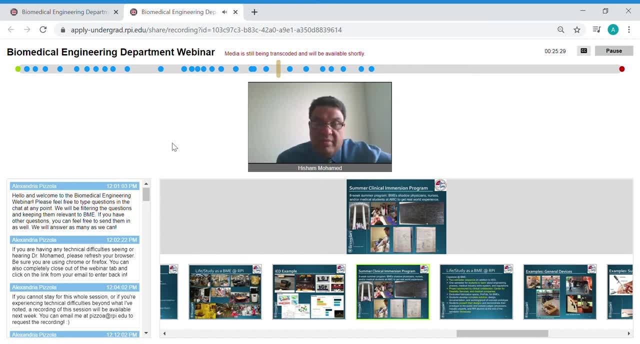 they meet with their. they meet with a doctor at Albany med. They meet with them at the end of the day and they meet with them once weekly to talk about the procedures and talk about what they have seen And they have learned. they write their ideas in a notebook so they can make. 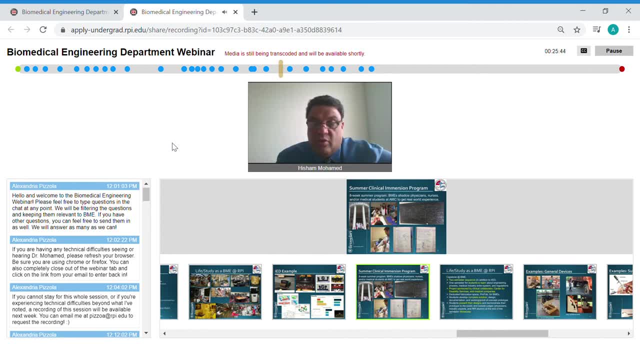 improvement on what they see or if they see anything that can require improvement, they write this. And the last week we put all these ideas, we researched some of them and we picked the winning ideas to move forward and use them in the capstone project or follow up on them. 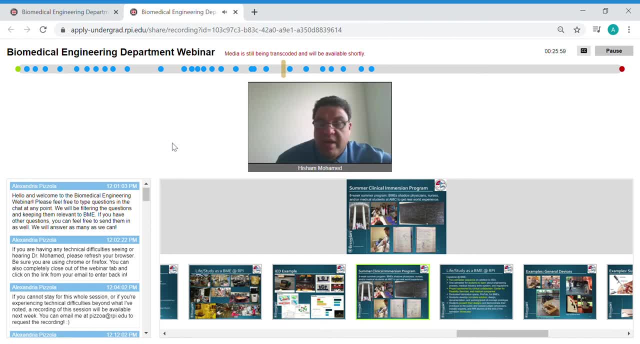 They very good experience on match, anywhere else where the students pre-med, or the engineer, the bachelor one get an idea, some of the pre-med one. after they did this they said: I'm not sure I want to be a medical doctor. 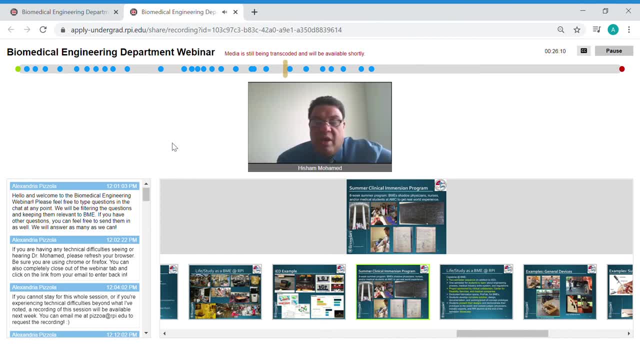 I don't. I'm not sure that is what I want to be doing every day, And maybe I will focus on being an engineer and vice versa. Some engineers said I will. I think I would like to cross the and go to the other side, where I will be a doctor versus an engineer. 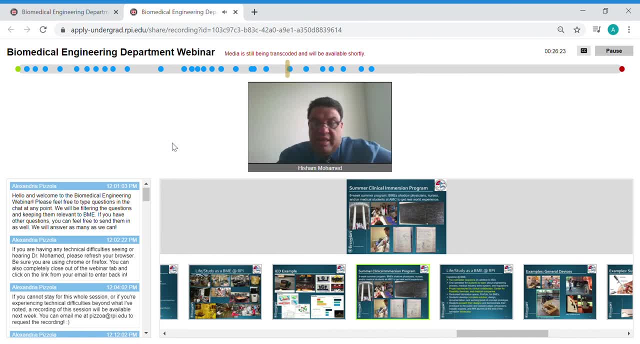 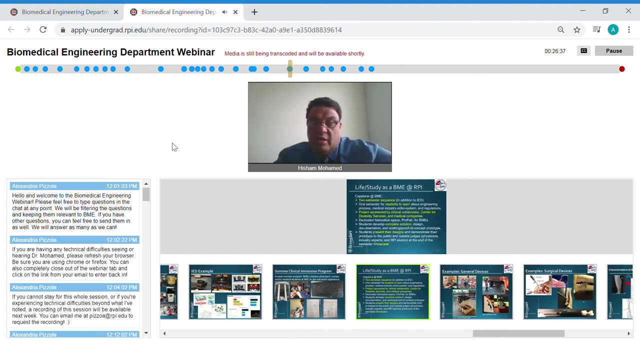 very valuable program. I don't think there is anything similar around the nation, and the one the clinical immersion program that are around that exist are very expensive for the students, So it's a very good experience for them to get this last thing that we are proud. 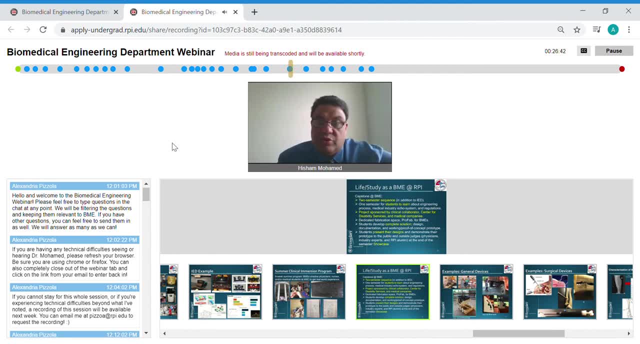 of is the. the our capstone at RPI is a two semester capstone. In addition to the IED, students learn about the process, medical industry. They learn also about the regulation. They learn about the actual property, patent, Some of the laws that are relevant to what we do. 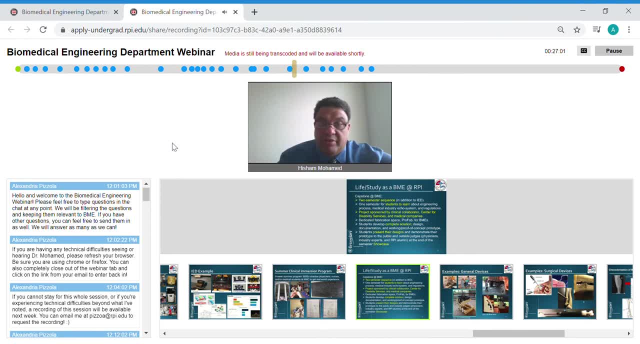 They have all the projects sponsored by clinical and by industrial collaborators, medical companies, So they interact with experts in the field. They get a, they get to work on a real problem and make a solution that's that somebody will use or will follow up on. 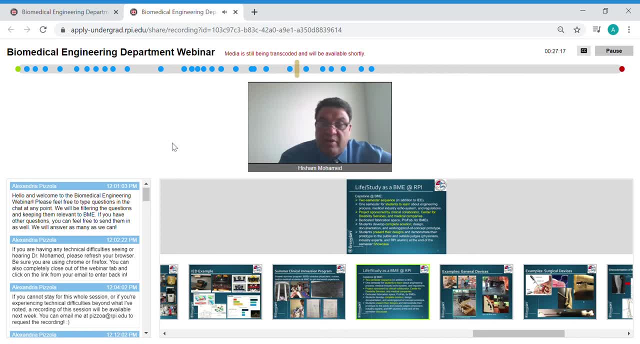 They have their own fabrication space. They develop a complete solution at the end along the way They designed their. they present their designs at different location, a different occasion, sorry, And they have to maintain documentation as if they're going to submit to the. 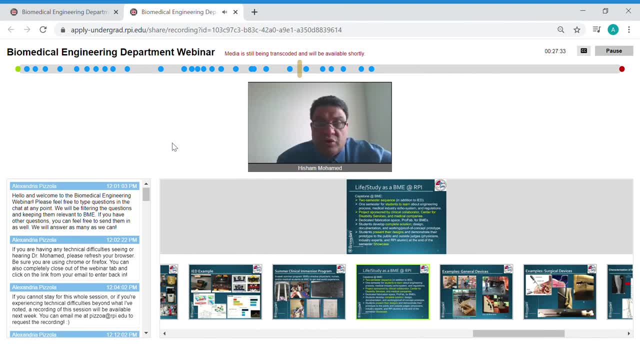 FDA, So it's a very good experience for them. They go through the entire process Once they know what's expected from them and they know what a designer means. even that a designer needs to know a little bit about IP law or patent law. 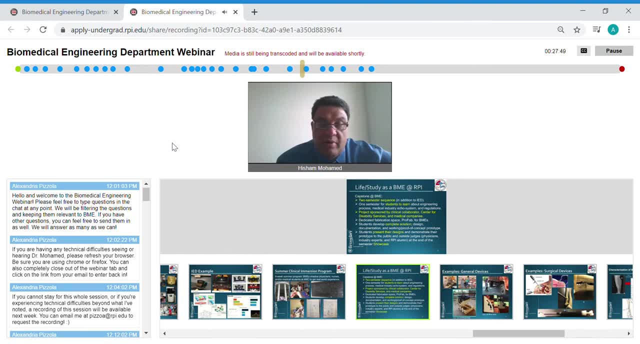 needs to know a little bit about the FDA regulation. They know to know about reimbursement, how how hospitals get the inverse for their, for their procedures, So they can be a better designer at the end of the day. They they know when they're working in this environment. 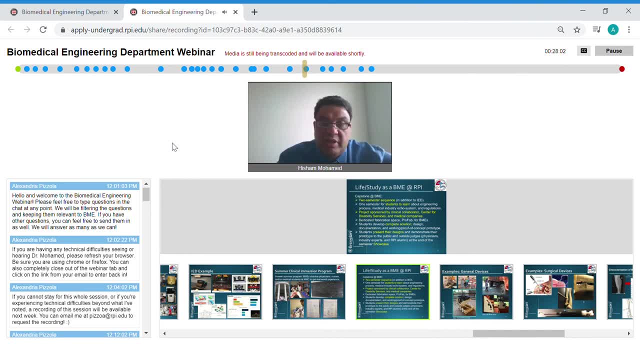 they understand what all the parameters that exist there and make sure that the design is the best solution that can come out with us. So that's something that we're very proud of, And I will show you a couple of examples from from our, from our capstone. 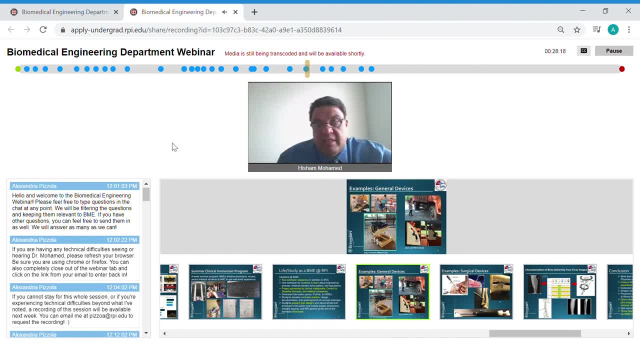 So we work closely with Albany center for disability. This is a center that deal with all the disabled kids in the area. They have all kids from all shapes and all spectrum of disability And one of the problems that they have is their dentist on site. 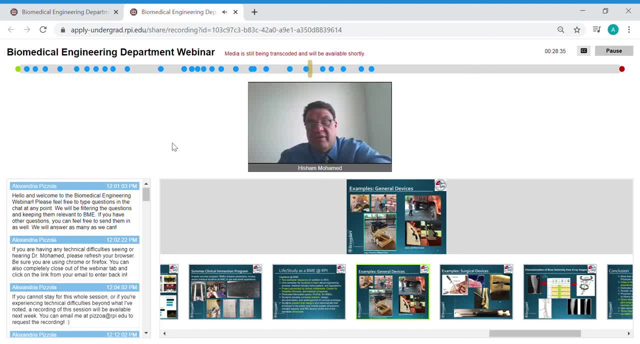 They have a problem because every kid has a different wheelchair. They are none of them standard, different sizes, Some of them have different mobility problems, different cognitive handicaps, And so you can see the dentist has to sit on their knees, has to. 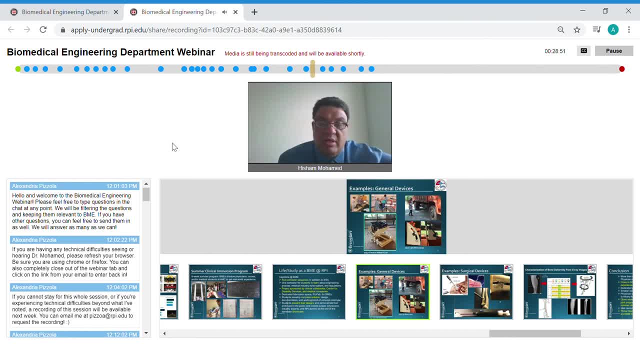 you know has to play acrobat to be able to provide regular dental treatment for these kids. So they ask us to have a dental chair that can accommodate any wheelchair and can still do all the function up down tilt that the dentist can do without. 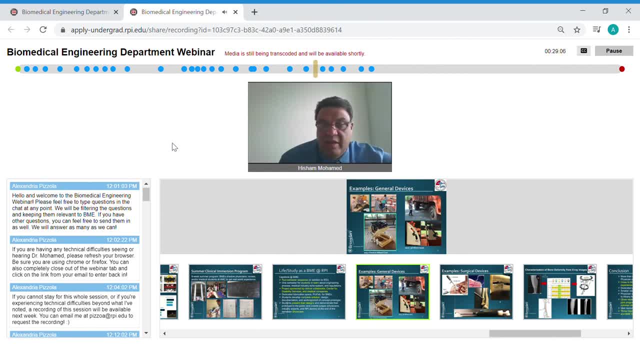 you know, without them being putting strains on their back and stuff like this, And we designed a solution for them and they were very happy with it. The other one, it was a cane that will help a vision impaired person to- not just to- 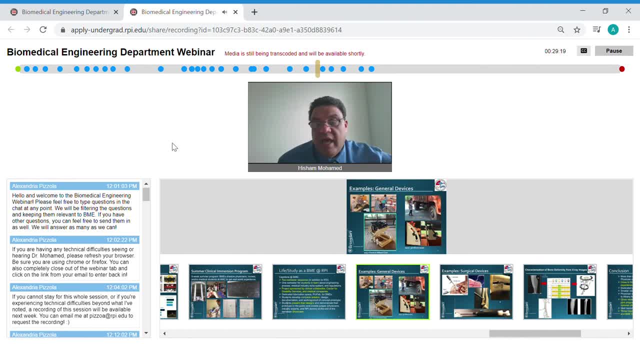 you know, tap on the ground and see what the obstacles on the ground level. but to help the patient almost see what's around them, We send a series of sensors that can tell them if the obstacle is high, like the one on the seat on the truck here. 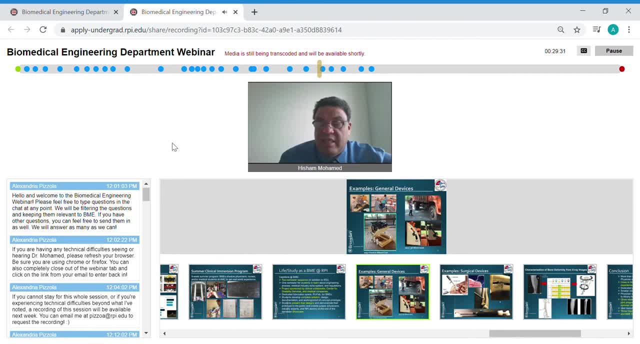 it can. also, it was meant that in the future it can read signs and tell them what's surrounding them, and tell them there is a sidewalk, there is a store, there is X, there is Y. So as they're walking, they're getting information from their cane with a earpiece. 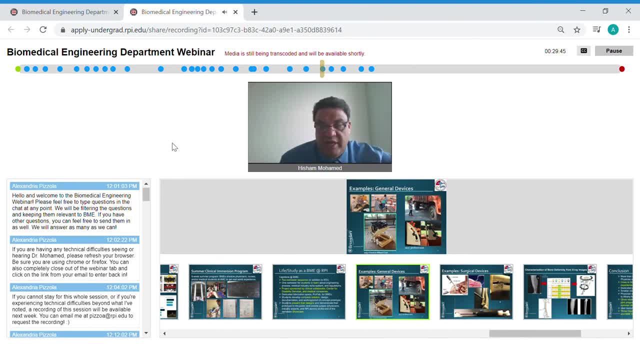 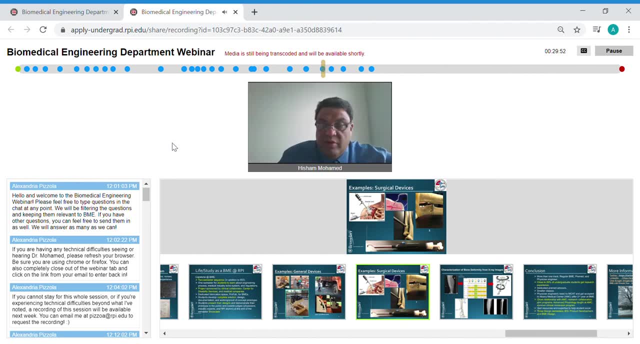 and that will have them to be to be safer and to get more function out of it. There's another project for a surgical device. You can see we took a surgical device that you see in the bottom. the black part is original part. 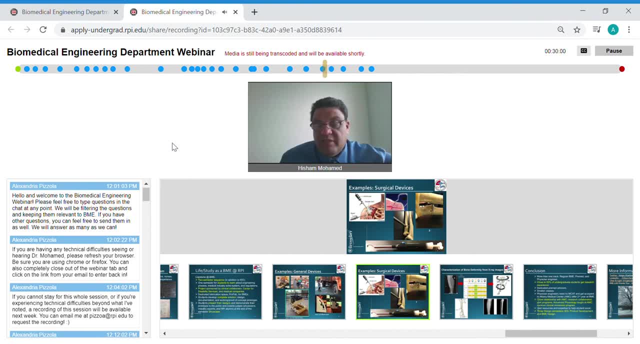 The white on the right is: we took the gut out of this. the surgical piece to be to do our own. This is a surgical piece meant for doing suture when you are doing orthopedic surgery and you cannot see on the other side. 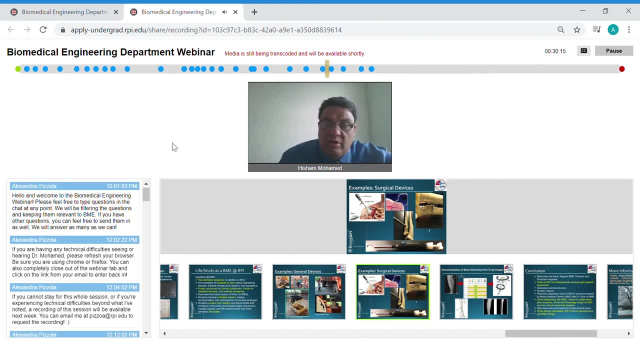 if you drill a hole in the bone and you'd like to do work on the other side, you can not do that. So this tool help you doing that And it has some limitation and we took the original tool and we were able to modify it and make it easier for the. 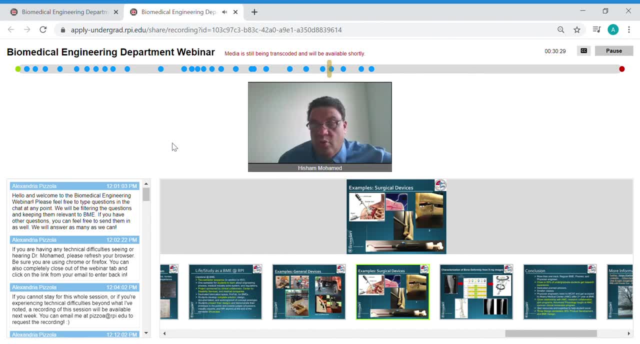 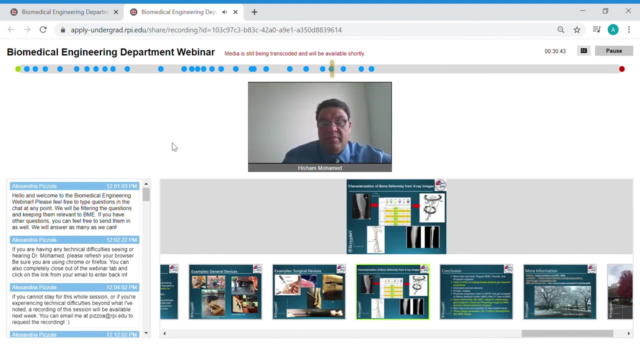 for the surgeon to work with it and requires only one hand, instead of having two hands busy with one device and having some other surgeon help with the with the rest of the procedure. Another example of looking at imaging and automatically being able to assess what the break. 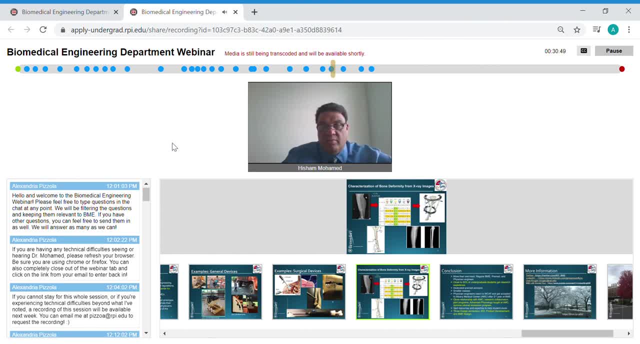 the damages in this case is a broken bone and the broken bone that are to heal this. their people are put in this device that will help them heal and bridge the bone to grow back to its normal length, And these devices requires adjustment daily or sizes and angle to make sure that the bone heals correctly. 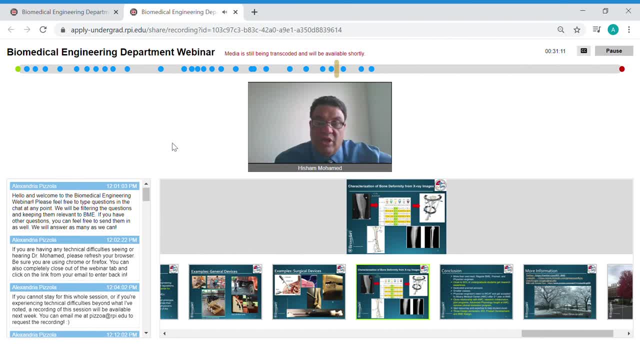 And this is usually. it's a plan that's made by a doctor and it's the implant. The putting this device is a decision made by a doctor, based on medical imaging, And some the problem that came to us was younger doctor and experienced doctors sometimes come to a different conclusion. 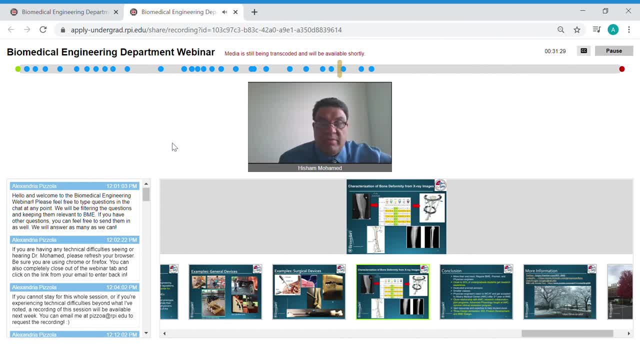 And sometimes the output of this is dependent on the doctor experience. So, instead of depending on doctor experience, we made this automated. so the then there is no. we took all the learning from experienced doctor and put this to make sure that the analysis of the images of a major degeneration of the treatment is automated and get the best output out of this treatment. 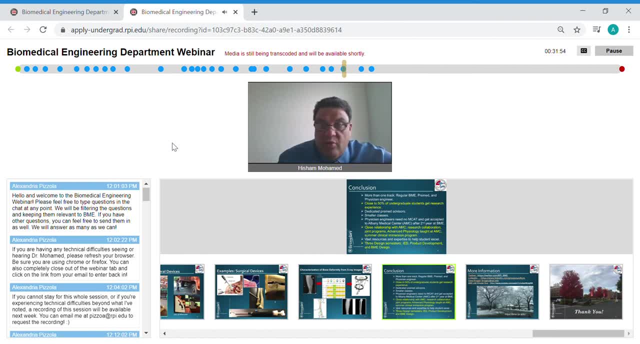 In conclusion, we have a flexibility. We have multiple track within the BME preparing people for, for the, for the future. we have, as I said before, we have a flexibility. We have multiple track within the BME preparing people for, for the future. we have, as I said before, 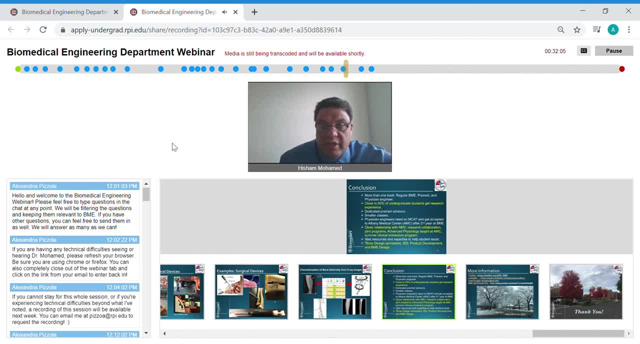 50% of our undergraduate do research. that hands on experience doing research that's in addition to the hands on experience that they get during their regular labs. BME lab biology lab. 50% of our undergraduate do research. that hands on experience doing research that's in addition to the hands on experience that they get during their regular labs. BME lab biology lab. 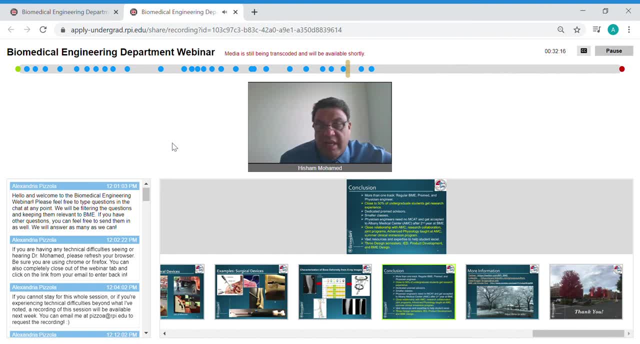 the advanced physiology when they treat animals and pigs and their work as IED and and capstone. We have dedicated premed advisors. Our classes are much smaller. If you are a physician engineer, you don't need to have cat, You don't need to have a cat. 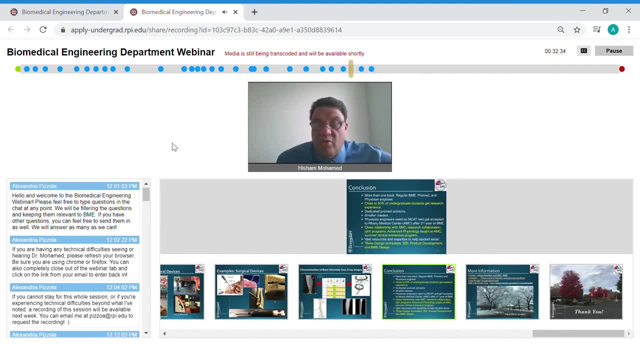 We have this and you can get to medical school easier. We have a very good working relationship with Albany Medical Center, which is about 30 minutes drive from where we are, And we have also a. we have also a relationship with Mount Sinai. Albany Medical Center is the one that teaches the advanced physiology. 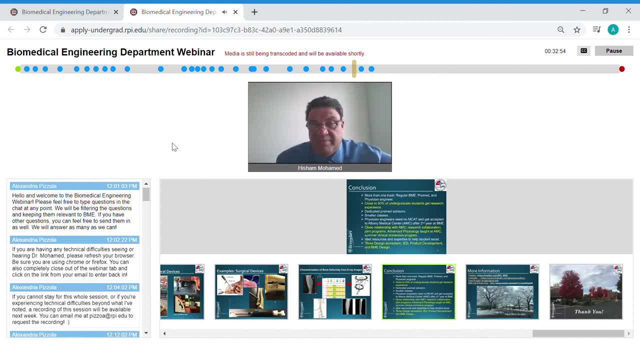 So they, the students, go there and get the class and get the hands on experience. They have tons of resources and expertise to help the students become better, Better designers prepared, better for tackling the workforce. And we have three design semesters to make sure that the students, when they hit the ground, they hit the ground running. 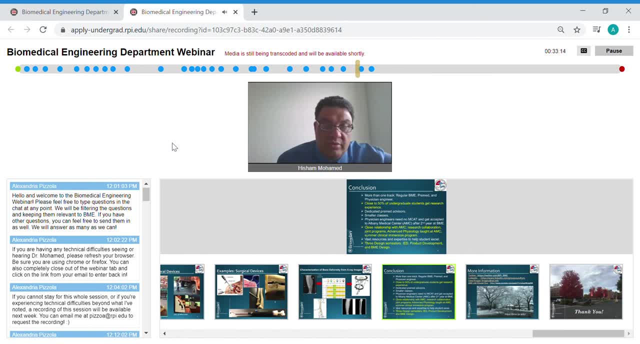 and they have. they appreciate and understand how things work professionally, But they also have an appreciation for continuing learning, because the education will not stop with their bachelor degree For sure. We are in a field that's fast moving, Technology is moving, and they have to learn, by time that they're leaving school, that they'll be learning. 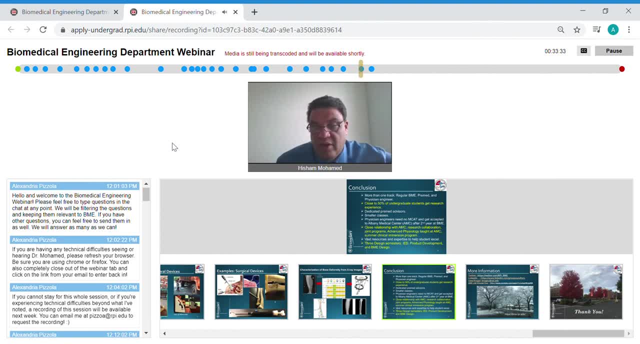 Most probably for them, rest of their life. so with that I will conclude my talk. I kept it good around the half an hour. that's good. there are more information that you can get on Twitter, LinkedIn or, just as I said, you can go to the web page of the department. 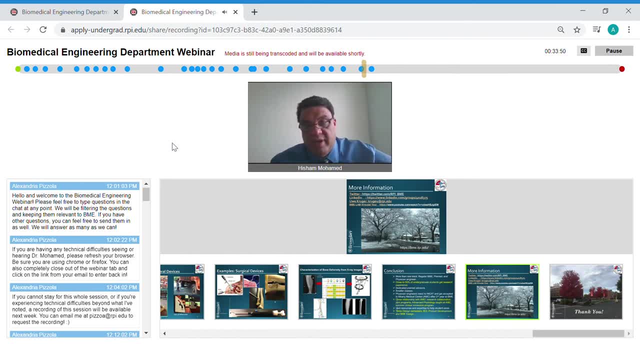 and find somebody to talk to. you'll find me there. you'll find department head there and other people talk to, plus the admission office. of course, they are your first go to. they will tell you what the best way to get your question answers there is also if we are on campus today, you would have. after this, you would have. 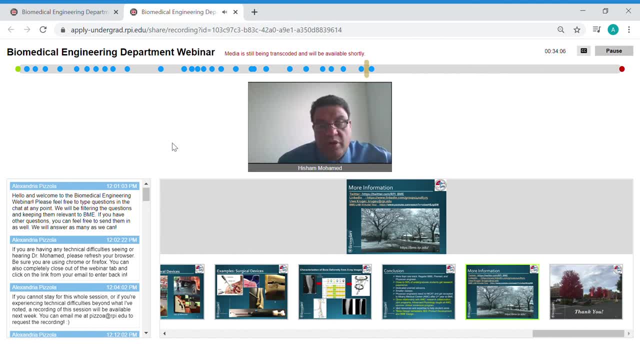 walked across campus to go and have a BME lab tour where you toured the biomedical engineering lab. unfortunately, because of the social distancing we cannot do that, but I put a link for the YouTube video where you can see five minutes tour of the lab, if you cannot capture this just when you go on YouTube. 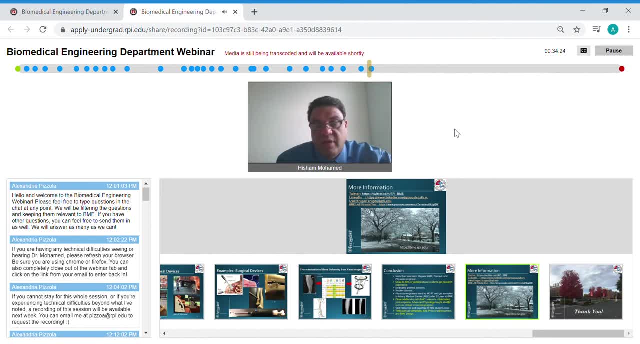 just search for BME, RPI, BME lab or RPI BME and you will. after a couple of clicks you should be able to find it and go through the lab to tell you what we do in the lab, and with that I think I will thank you. thank you for being.